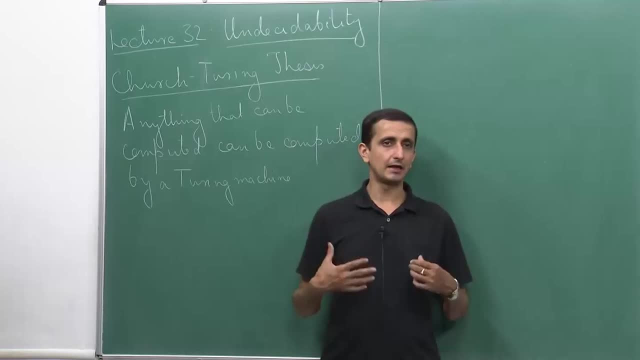 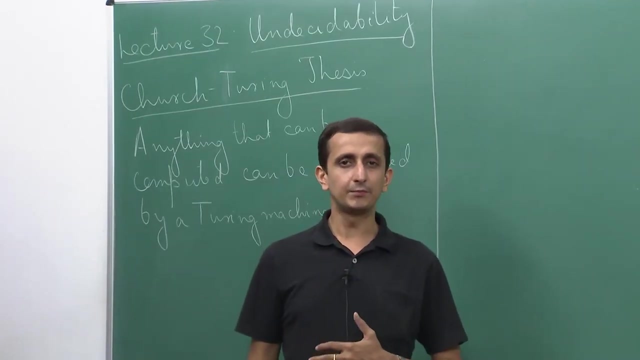 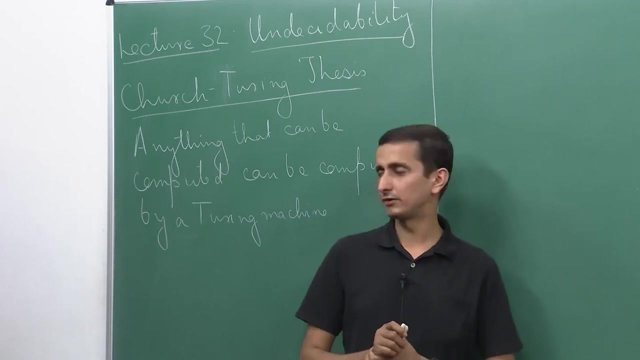 says, is that Turing machines are a universal. Turing machines can be thought of as a universal model of computation. So any problem, any computational problem which can be computed by any computational device, for that problem, there also exist a Turing machine that can decide that problem, If we represent it suitably in a language format. 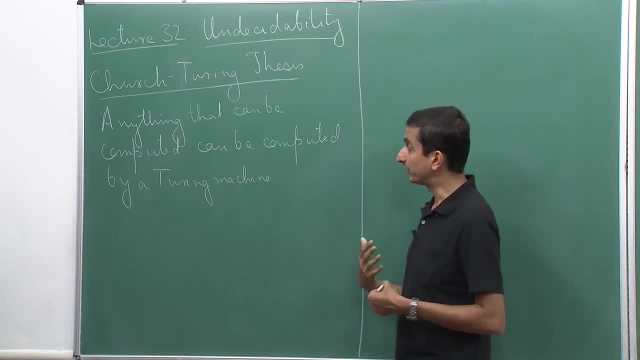 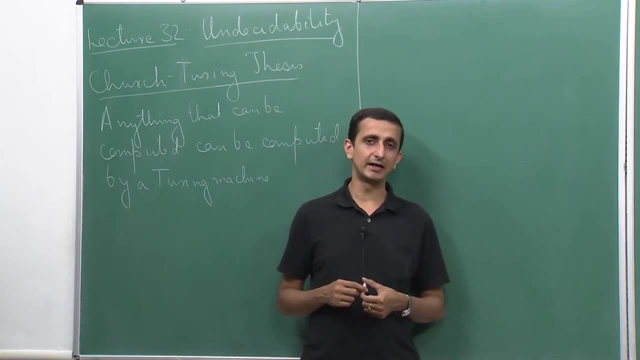 So basically, therefore, then, in the context of undecidability, what this means is that, suppose, if I show that a problem is undecidable, In other words, if I show that a problem cannot be decided by a Turing machine, It essentially means that it cannot be computed, It cannot. 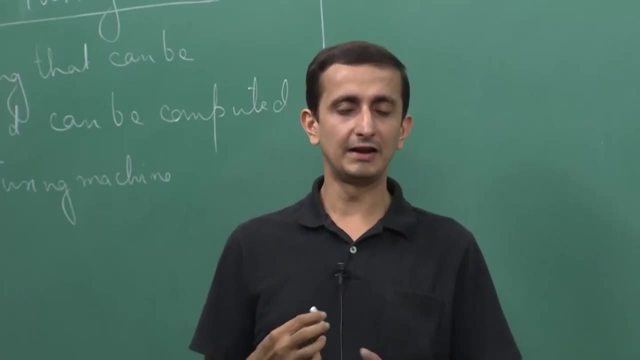 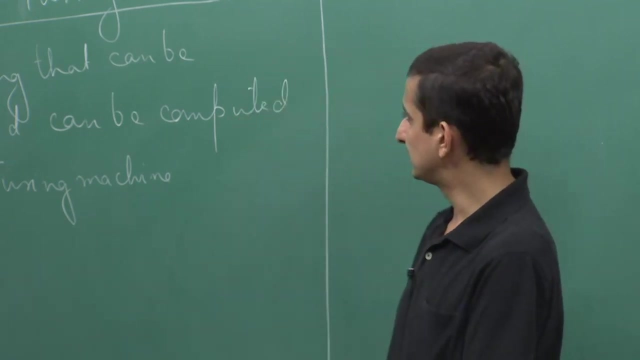 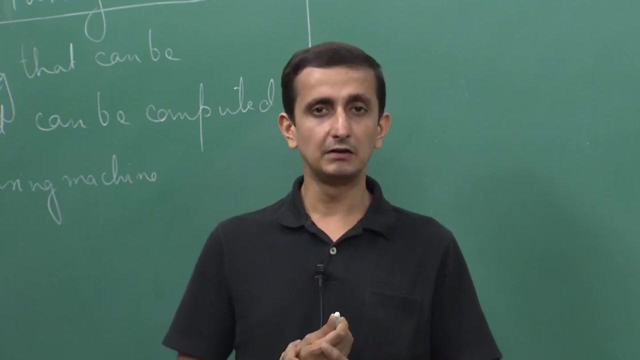 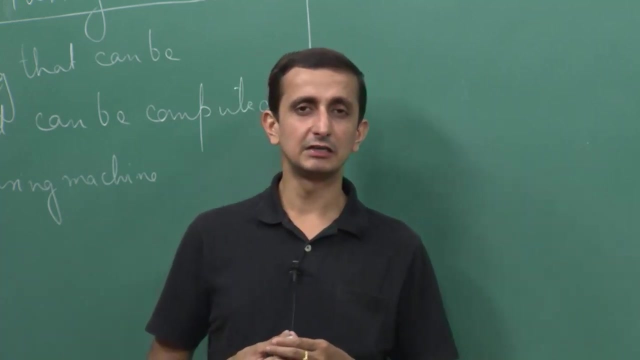 be determined by any computing model or any computing device that is available at hand. Okay, If you believe the Church-Turing theses. So this is actually to show that some problems are undecidable? is quite a big question, I would say, Because if you imagine, I mean with so much computing power that is available. 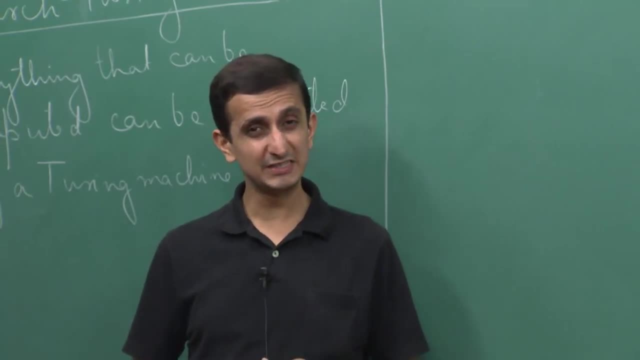 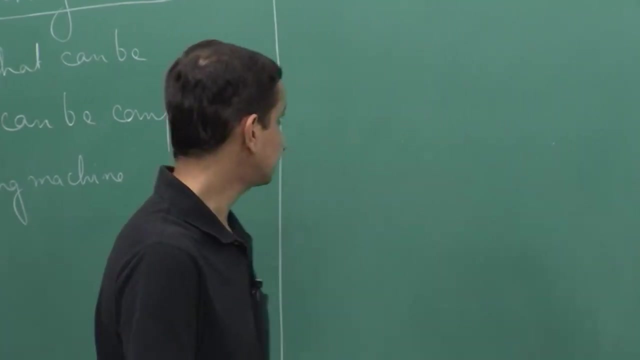 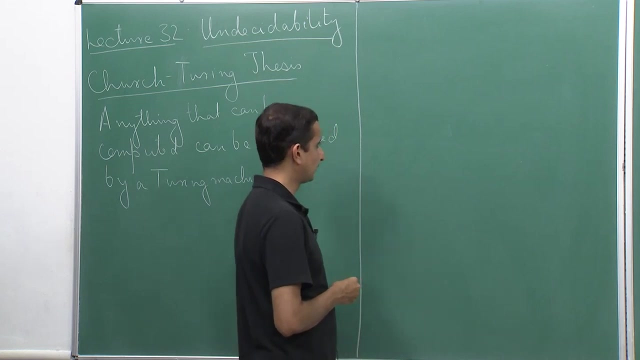 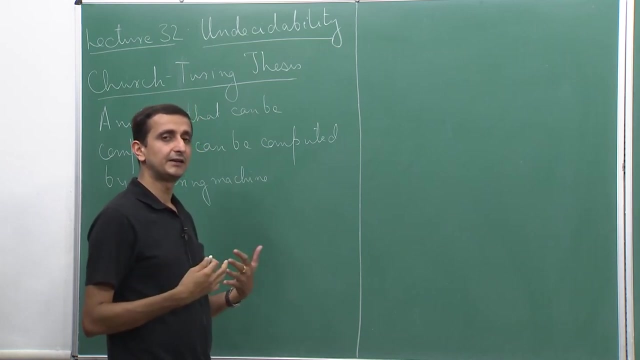 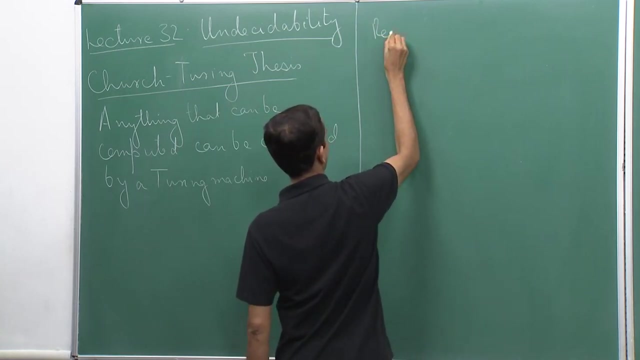 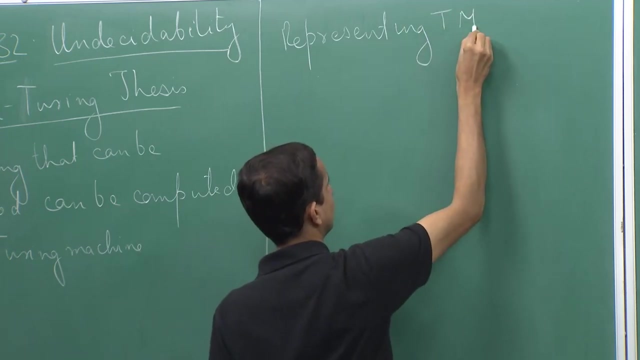 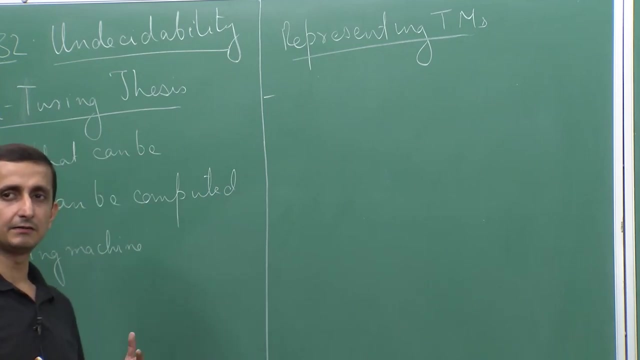 us today to say that there are languages which cannot be computed is something that is not immediately obvious. So before I show the first undecidable problem, let me talk about equivalence of Turing machines and so representing Turing machines by integers. So in our last lecture I said that any Turing machine, or, for that matter, DFA, PDA, you can. 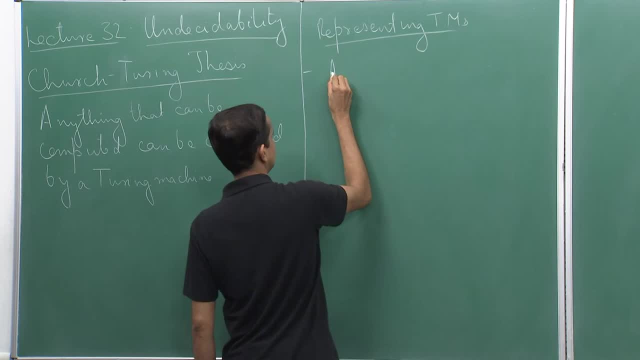 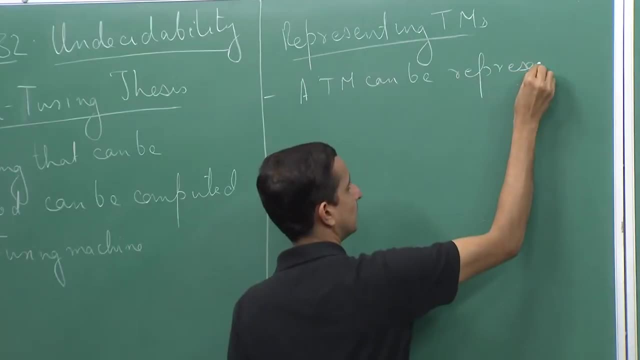 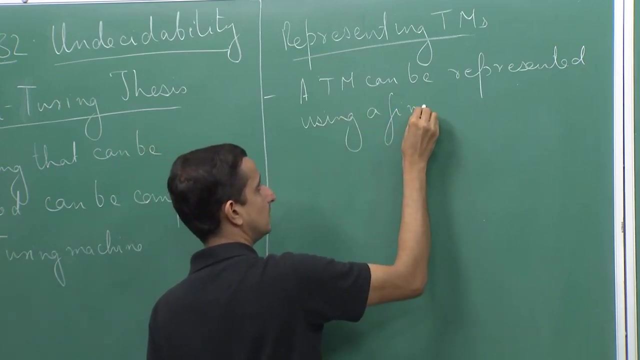 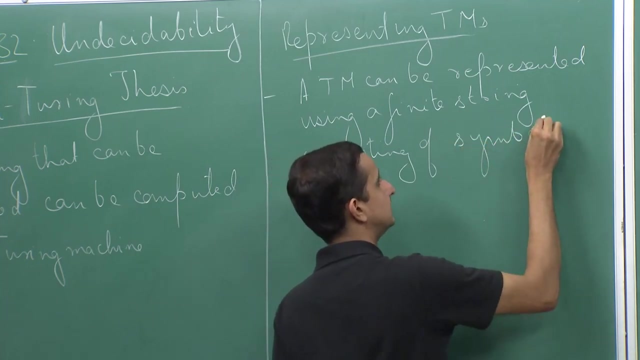 represent it using a finite string. So a Turing machine also can be represented using a finite string consisting of symbols which are not actually finite. So a Turing machine also can be represented using a finite string consisting of symbols which are not actually finite. So a Turing machine also can be represented using a finite string consisting of symbols. 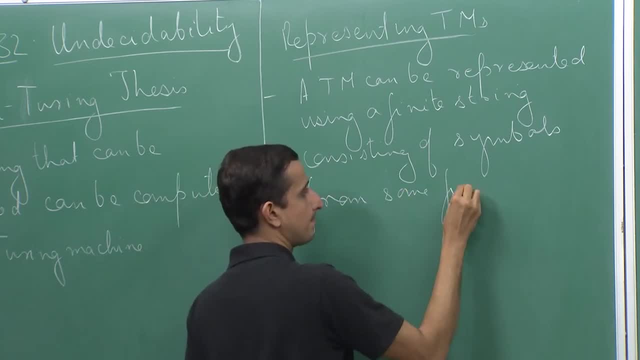 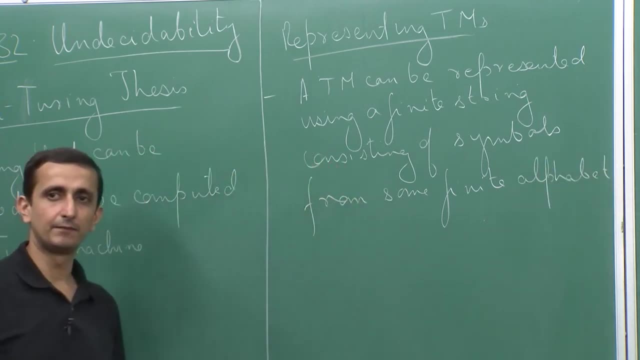 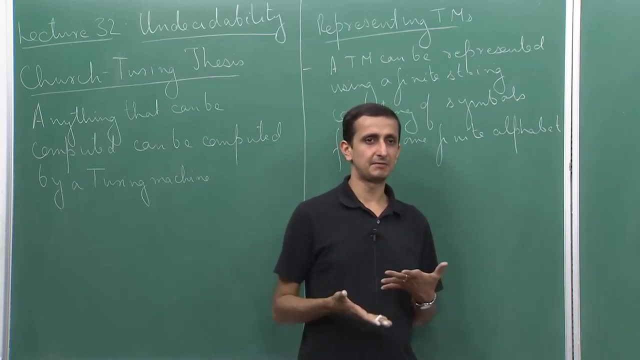 which are not actually finite. So a Turing machine also can be represented using a finite string consisting of the singular alphabet from some finite alphabet. For example, if I just represent the description of a Turing machine, that is the transition function: the states accept state, reject state. it is basically a finite string over. 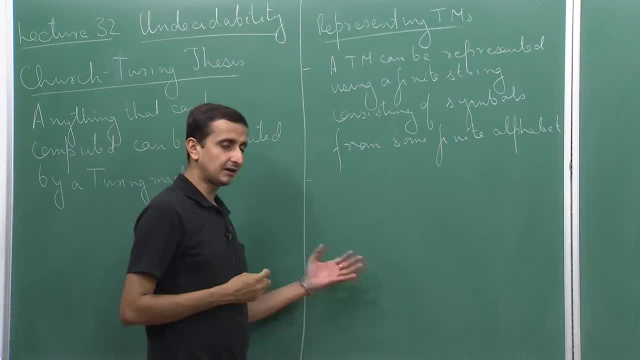 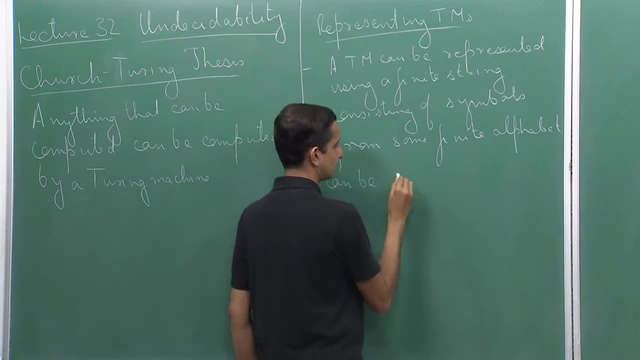 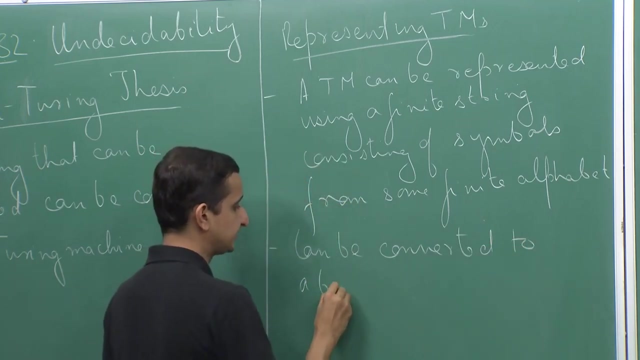 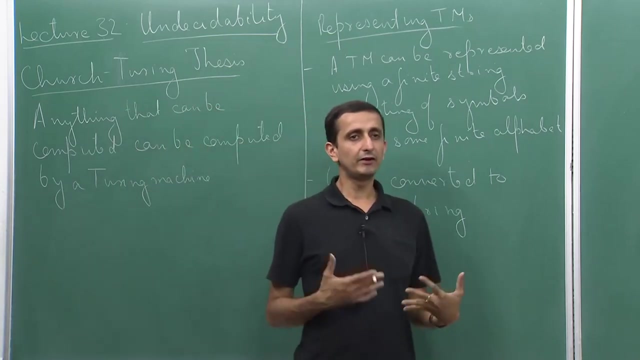 some finite sequence of alphabet. Now I can convert this this to a binary string. So what I mean by this is that I can take the string which represents a Turing machine and I can convert it into a string over 0 ones. The way to do that is: 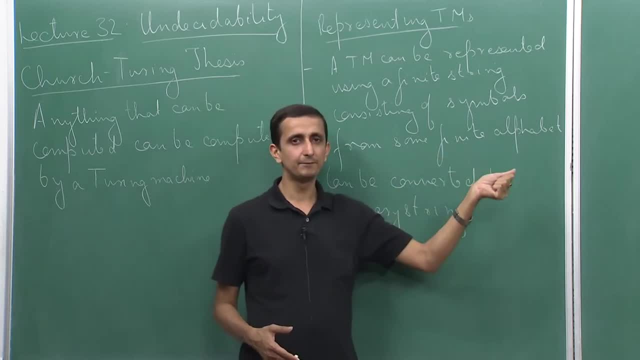 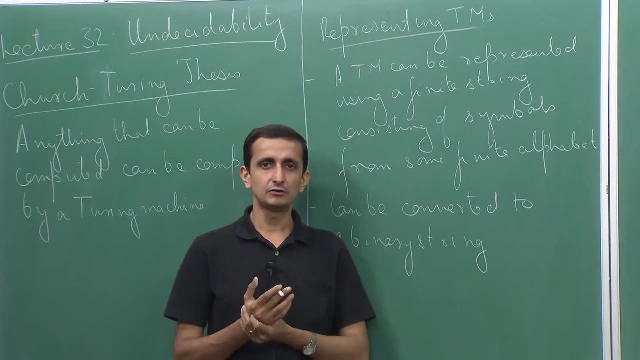 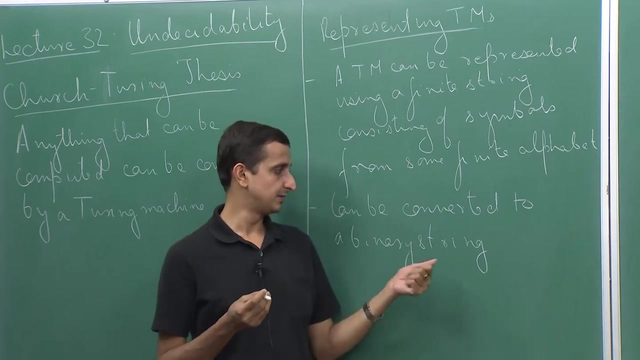 suppose I have a string over an alphabet which has size k, So there are k symbols in the alphabet. k can be any constant. So therefore to represent, I use log k bits over 0, 1 to represent each symbol of the finite alphabet, For example, if there are 10 symbols in that. 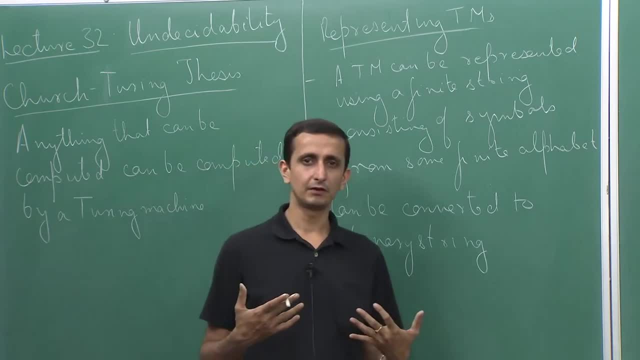 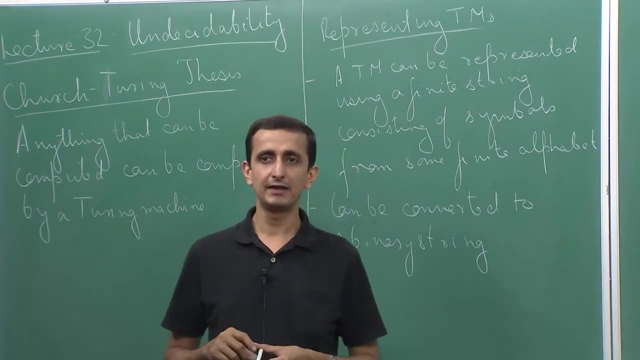 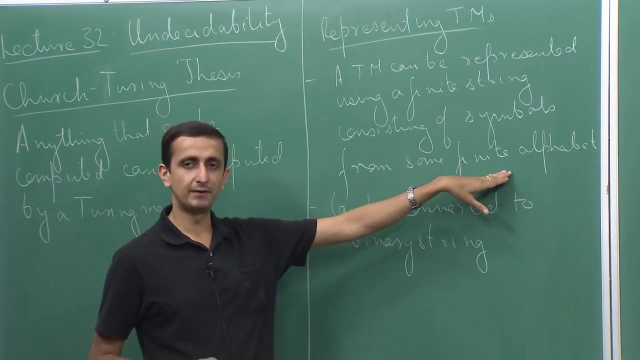 alphabet. I will use log 10, I will use the ceiling of log 10, which is basically 4.. So I will use 4 symbols. So each symbol of the alphabet will be represented by a binary string of length 4.. Now, therefore, I take a string over the first alphabet and convert it into: 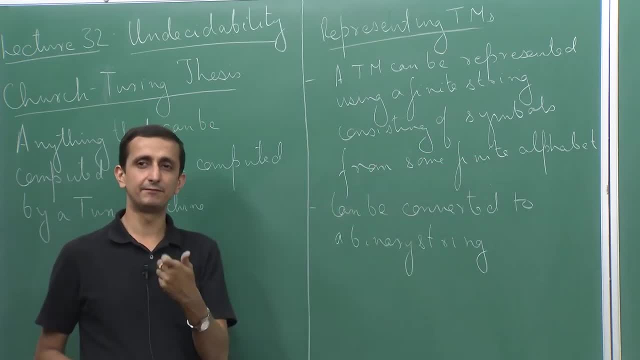 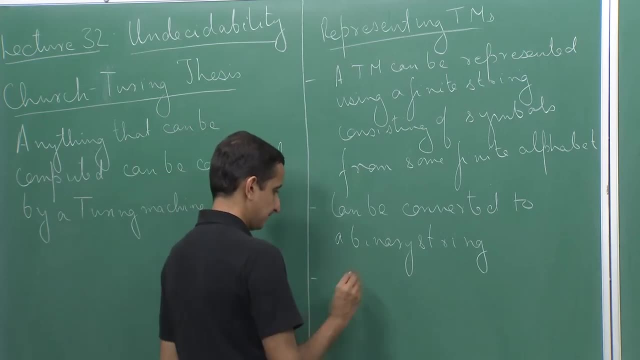 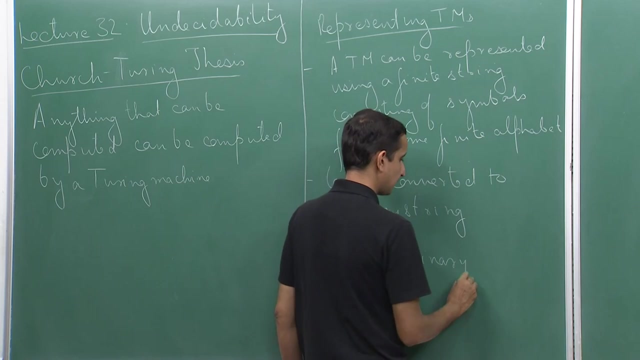 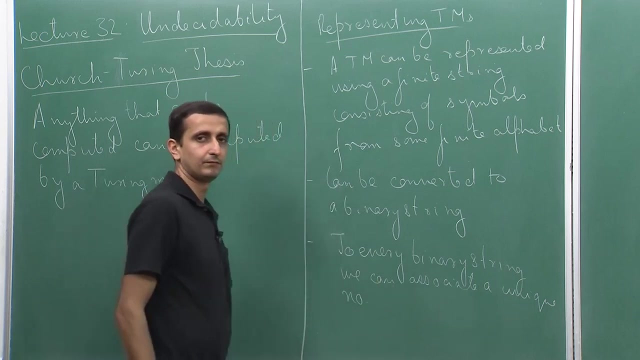 a string over 0 and 1, by replacing every symbol with its corresponding binary string. Now, to every binary string we can associate a, a, a, a, a, a, a unique number, So every binary string. so suppose, if the string does not begin with. 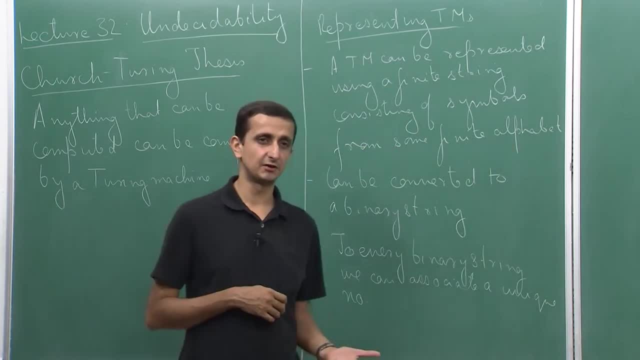 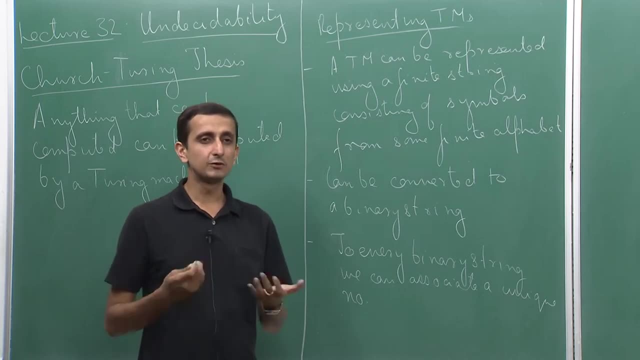 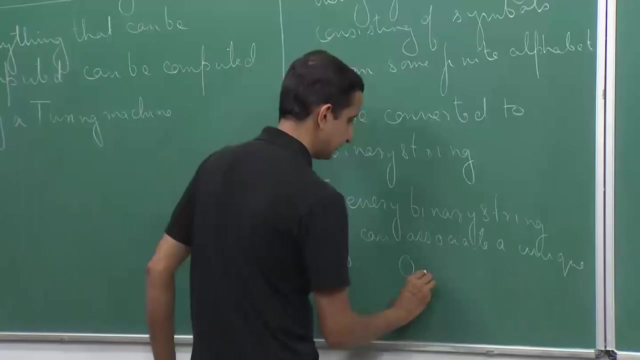 a 0,, then of course every binary string can be converted into its corresponding decimal string, and that is a natural number. But suppose if I have preceding 0s? so for example, if I have a string, let us say 0, 0, 1. 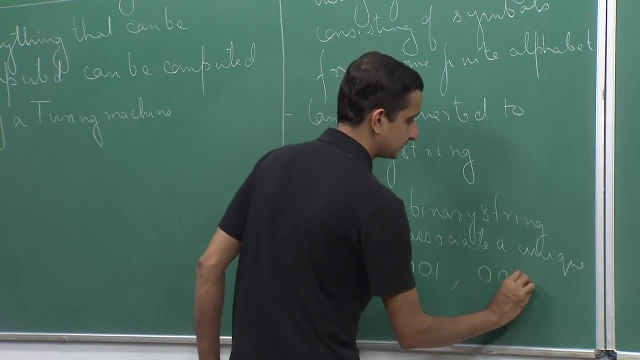 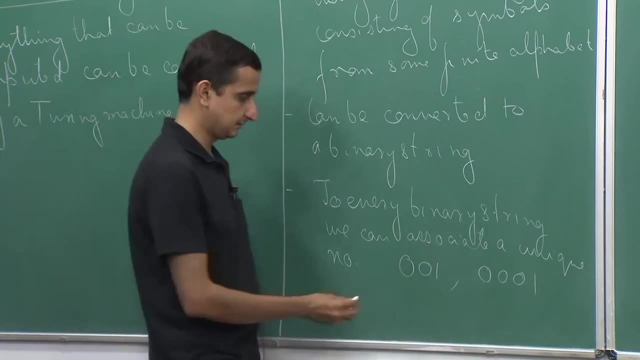 and another string 0 0 0, 1.. So both these strings, when converted to decimal, corresponds to the number. let us take a little bit more. let us say I have a string 0 0 1, 0 and I have 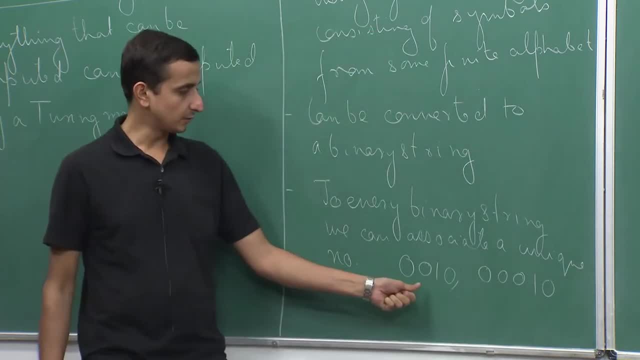 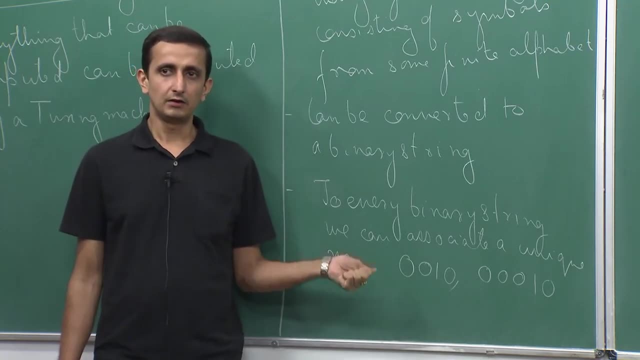 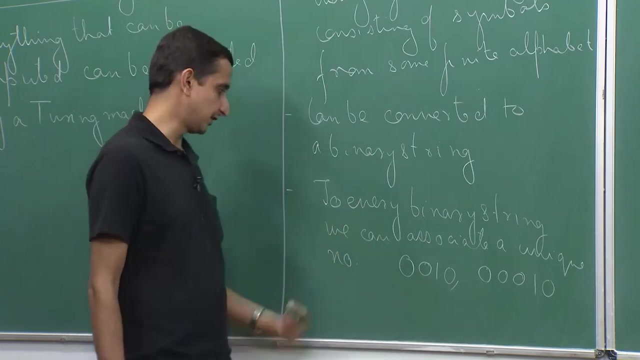 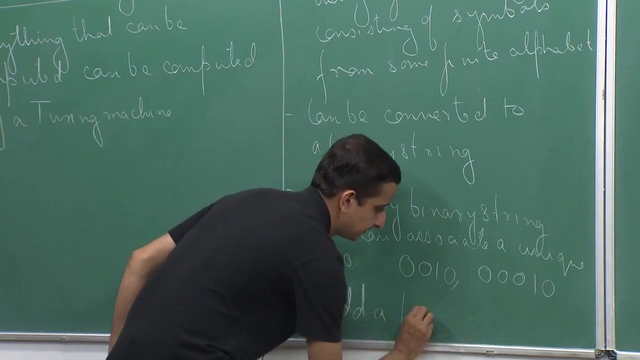 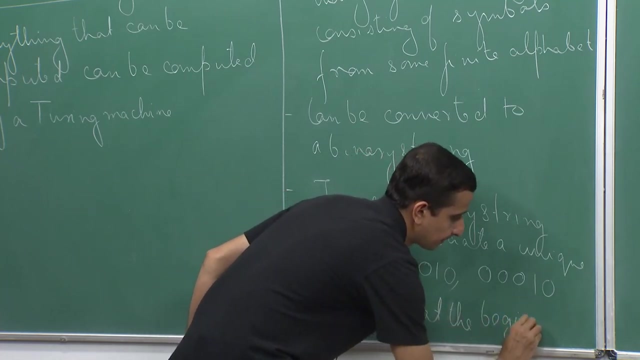 another string, triple 0, 1, 0.. So when I convert both these strings into a decimal, it corresponds to the number 2.. So to avoid this kind of a situation where two binary strings can map to the same natural number, what I do is that I add a 1 at the beginning. 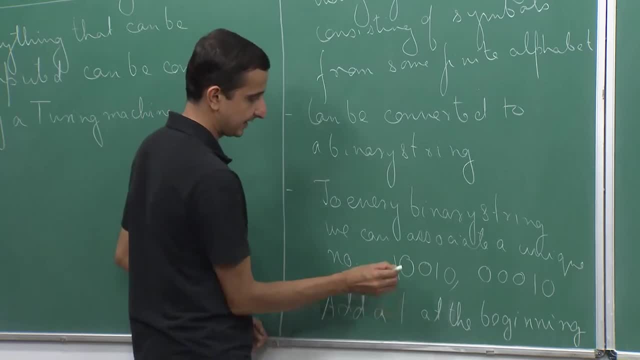 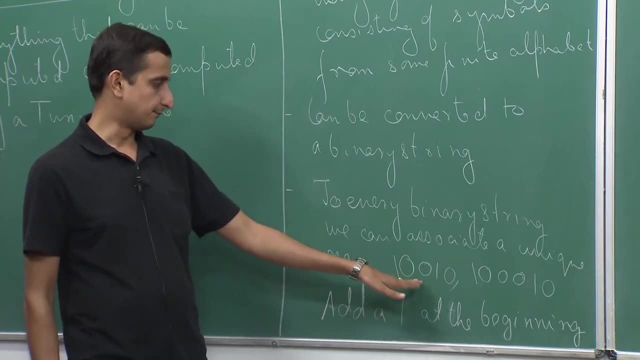 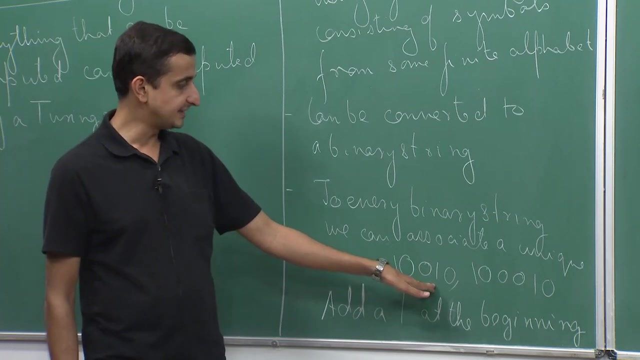 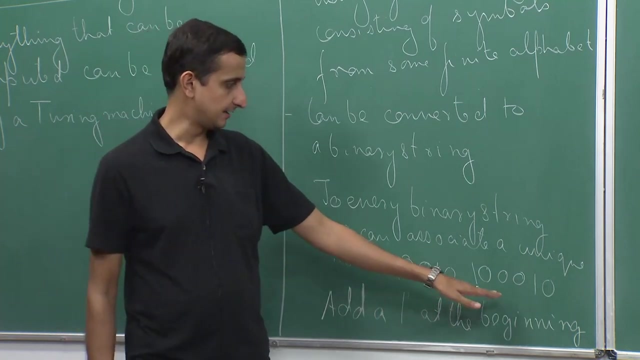 So now, if I, for example, add a 1 to the beginning of every string, so I add a 1 here and I add a 1 here, so this string now corresponds to some number. so in this case it corresponds to the number 18, and I think so. so this will correspond to 18 and this will correspond. 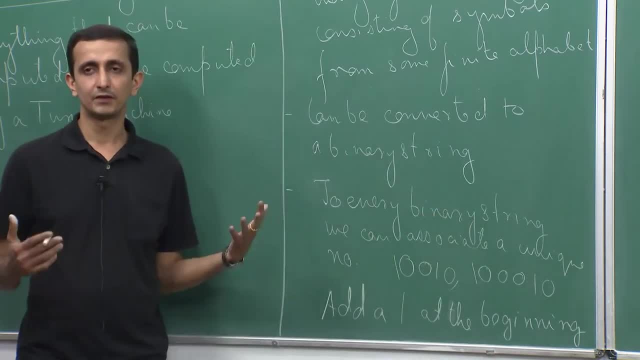 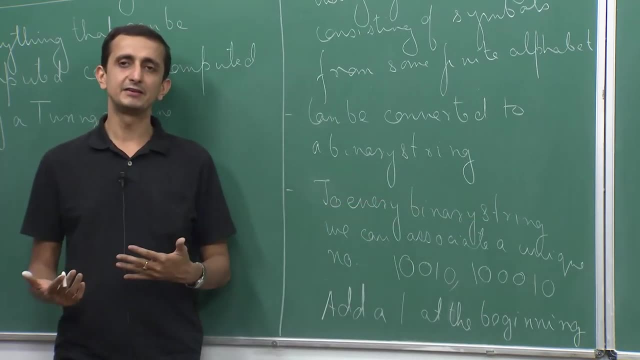 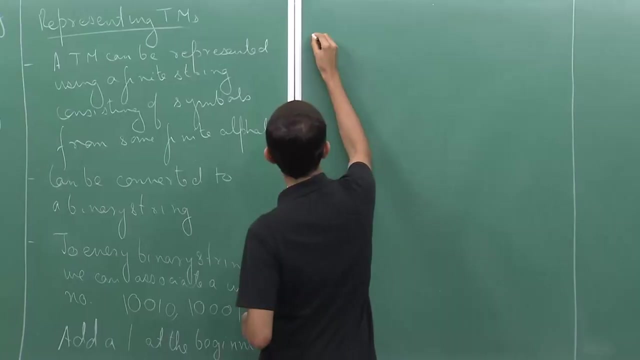 to 34, so they correspond to 2 different natural numbers. So basically, if I add a 1 to the beginning of every binary string, so I add a 1 to the beginning of every string, then every binary string corresponds to a unique natural number. 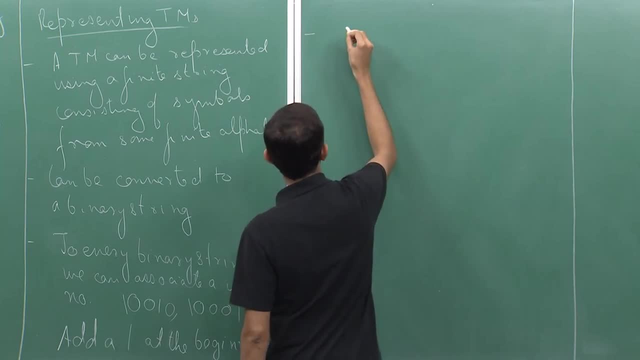 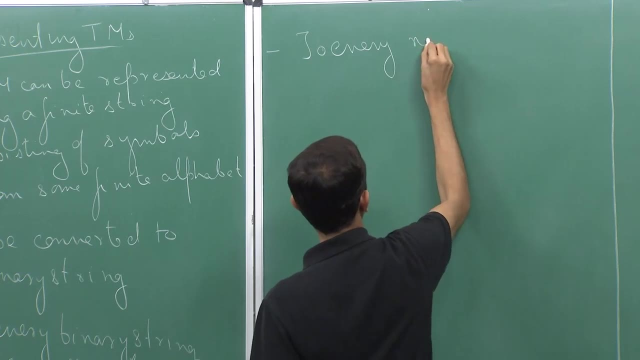 Now, to every natural number we have to add a 1 to the beginning of every string. so if I add a 1 to the beginning of every string, then every binary string corresponds to a unique natural number. So we can associate a Turing machine. 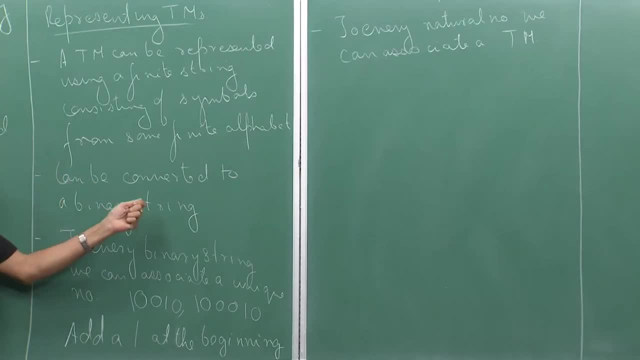 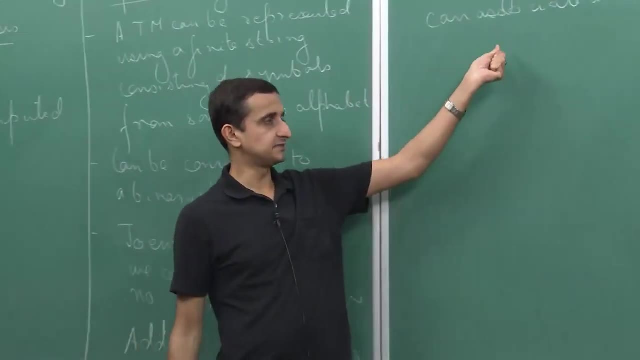 So by this mapping here, for every Turing machine I have a binary string which gives us a natural number. so there are certain natural numbers which correspond to a Turing machine, but there might also be some natural numbers which do not correspond to a fixed. 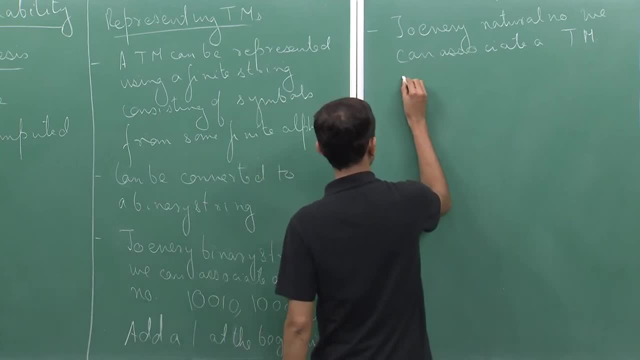 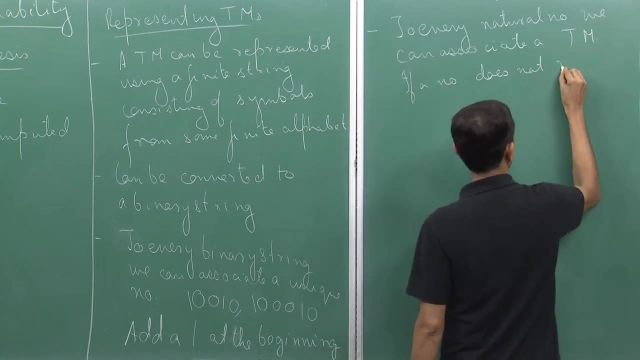 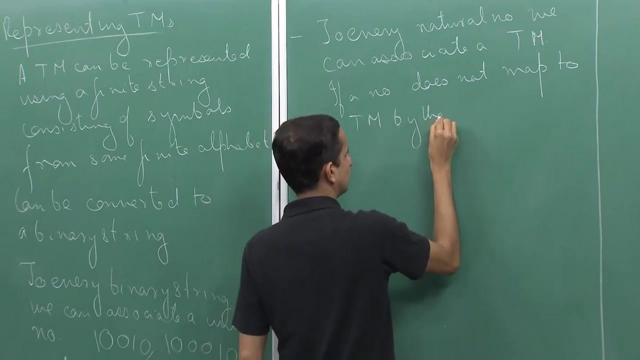 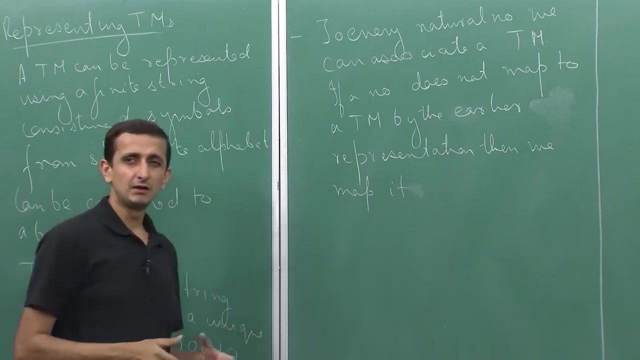 Turing machine. So what I do in that case? is that so if a number does not map to a Turing machine by the earlier representation, Okay, Thank you. Thank you. Then we map it to some arbitrary but fixed Turing machine. let us say a Turing machine. 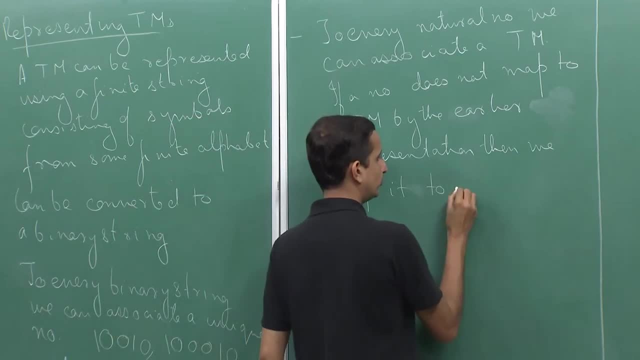 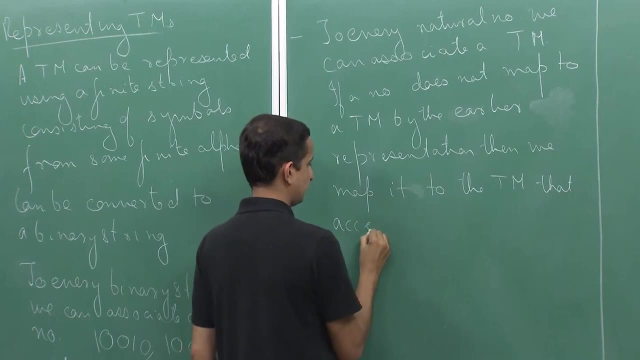 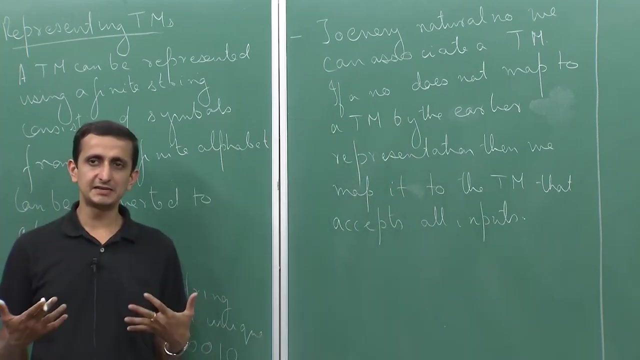 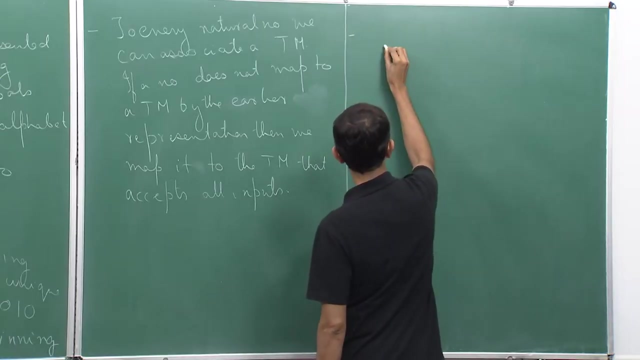 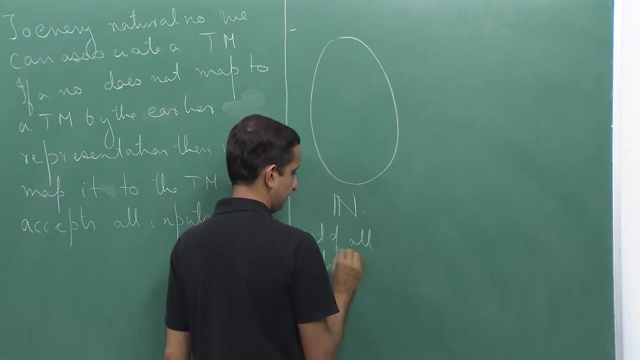 that accepts all its inputs, map it to the Turing machine that accepts all inputs. Basically, what is necessary is to have a function of the following form: so suppose, if I look at the set of all natural numbers, Okay, So this is the set of all natural numbers on the left hand side and on the right hand. 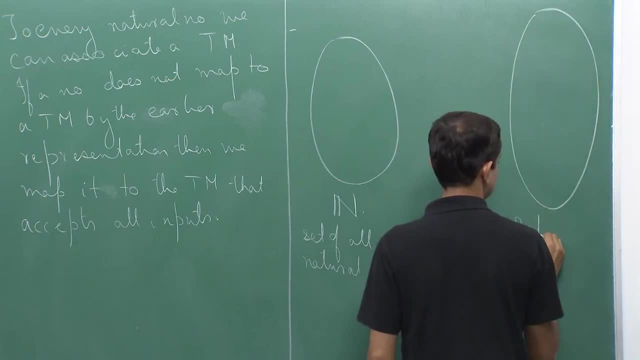 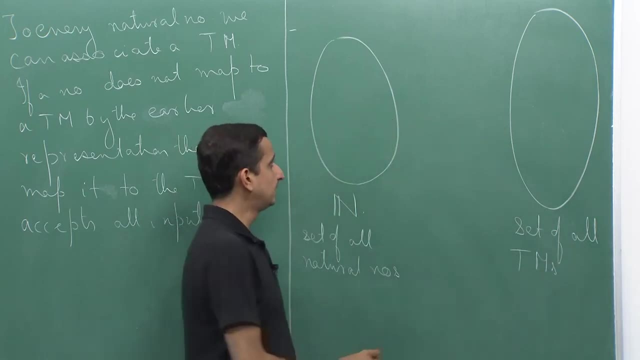 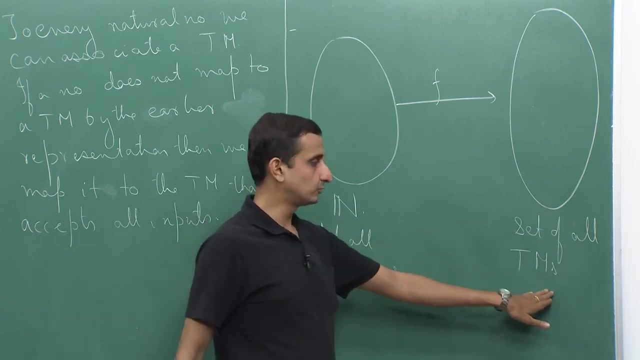 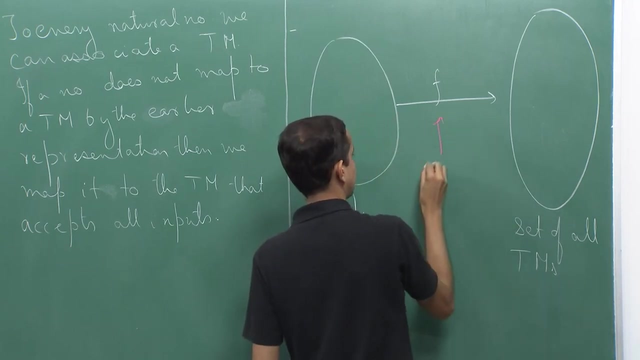 side. let us say I have the set of all possible Turing machines, So then I should have a function. let us call it f. Okay, From the set of all natural numbers to the set of all Turing machines, such that this f is a onto function. 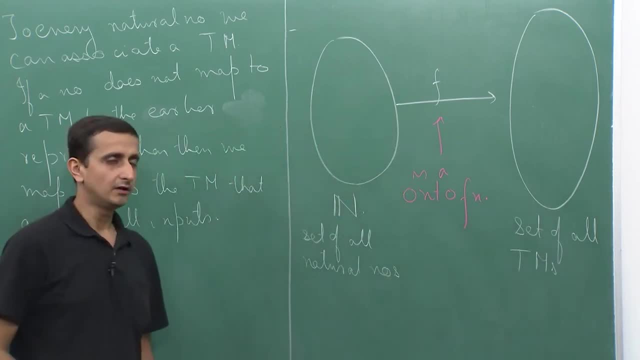 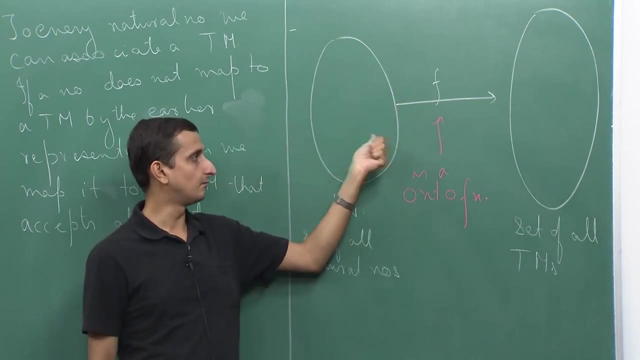 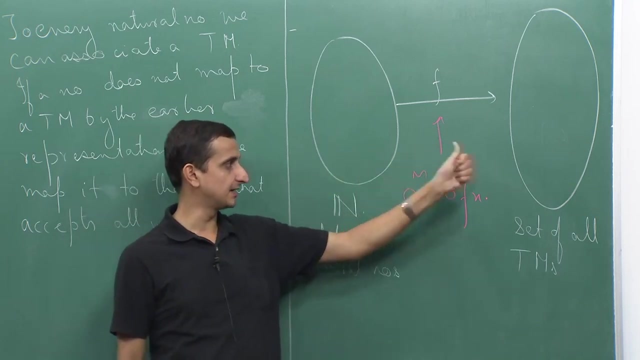 Okay, So, in other words, every Turing machine must have a unique. well, it did not have a unique, but every Turing machine must have such a function. Okay, Okay, So there is some pre-image. Okay, So every natural number gets mapped to a unique Turing machine and there is no Turing machine. 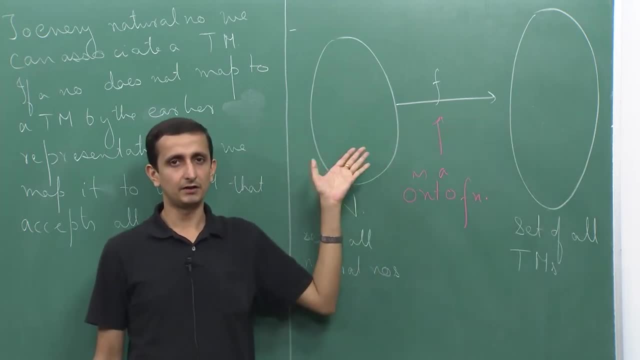 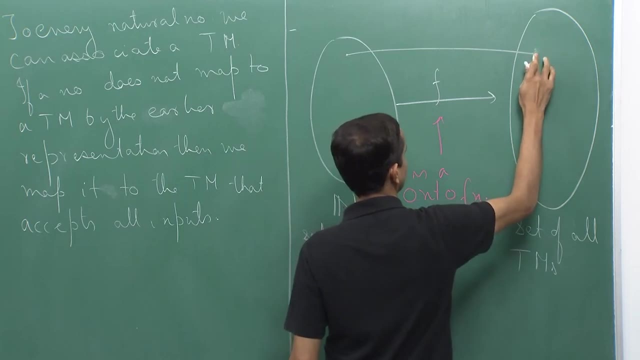 that is left out. there is no Turing machine that does not have a natural number as its pre-image. Okay, So, for example, I can map this to a number here, a Turing machine there, and I can map another number to the same machine. 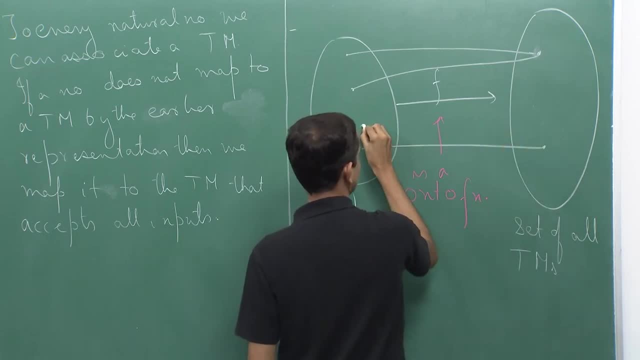 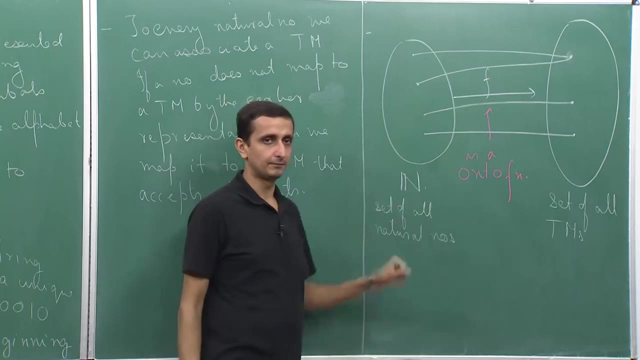 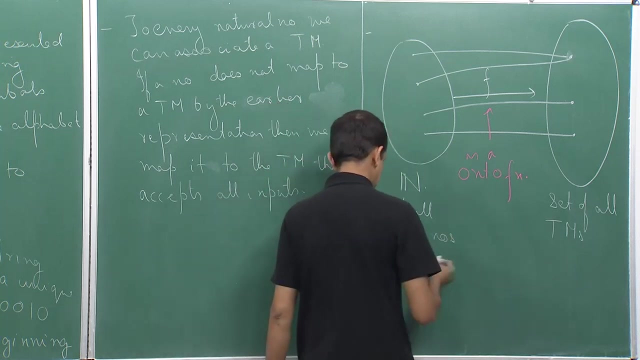 Okay, I can have a mapping here, something here and so on. Okay, What is important is that this is a onto map. So therefore, because I have an onto map, what I can do is that, for the j-th natural number, okay, we give the following notation: 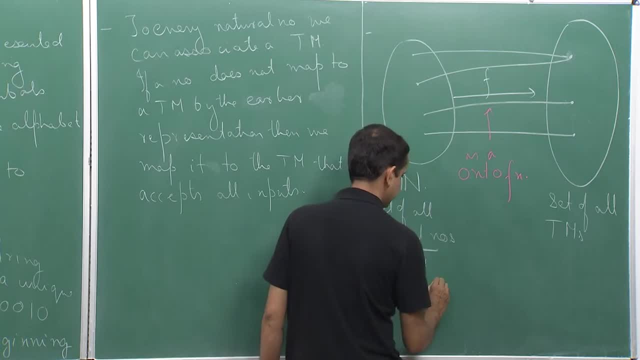 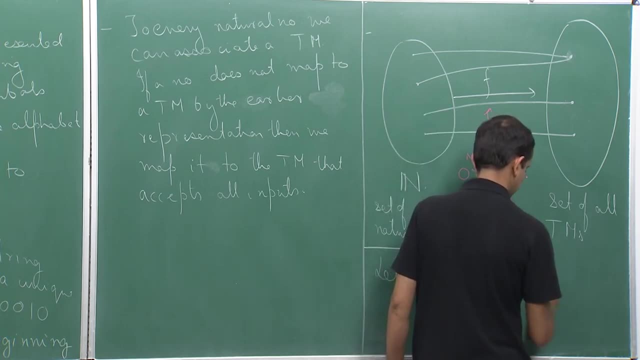 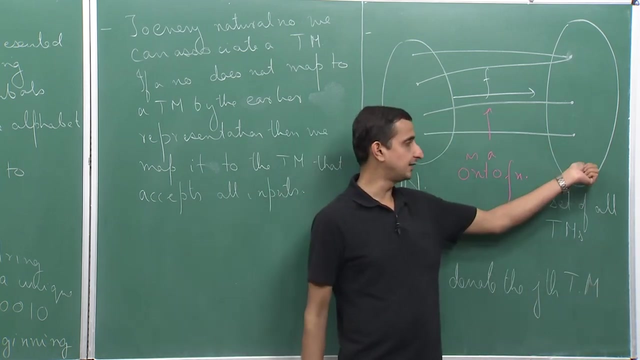 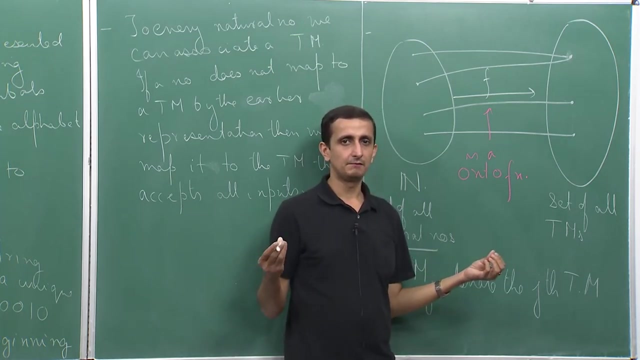 So let mj Denote the j-th Turing machine. Okay So, because for every Turing machine I have a number associated with it. Okay So, therefore, I can basically number all the Turing machines. May be that some of those Turing machines get repeated in the enumeration. may be Turing: 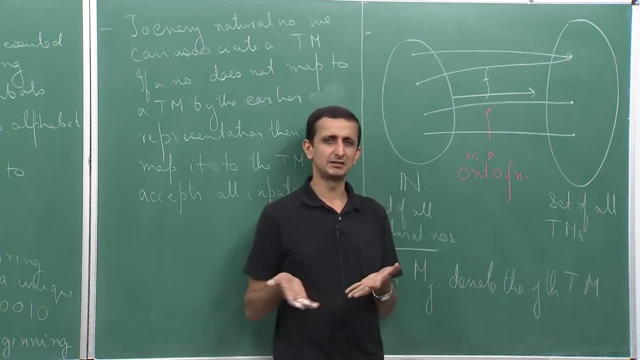 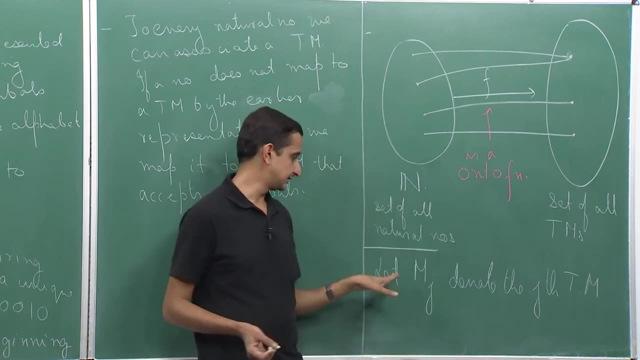 machine number 1 and Turing machine number 5.. But the same Turing machine. That is okay, But the point is that for every j there is a Turing machine mj. Okay. So this is very important. So this is number 1.. 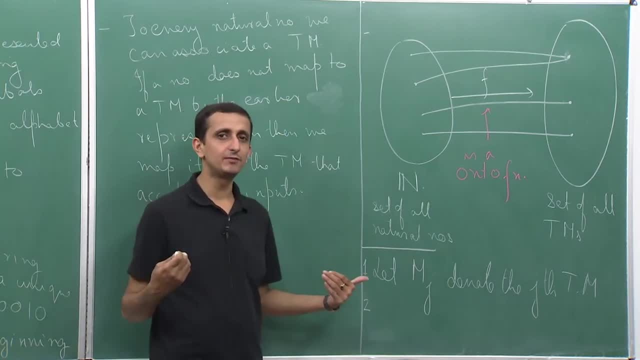 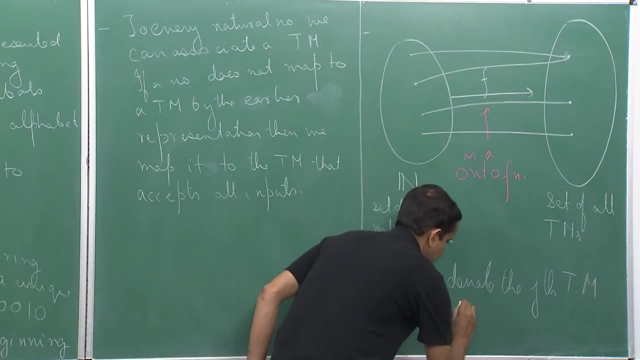 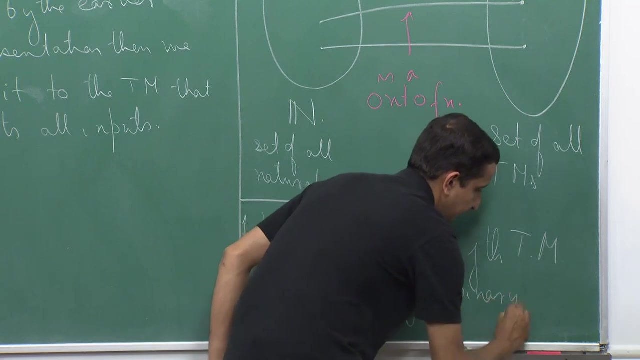 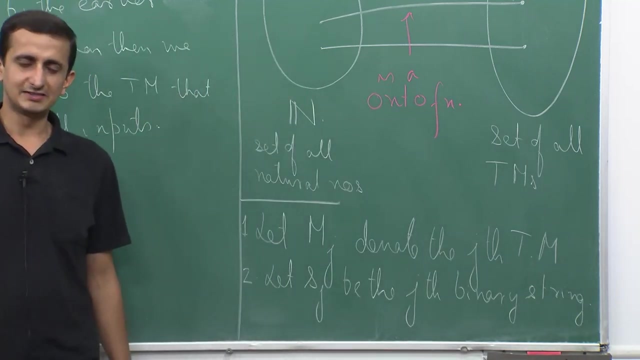 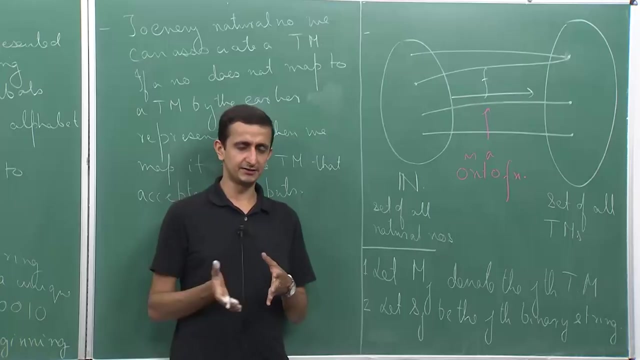 And number 2 is: I can obviously enumerate binary strings. Okay, So let sj be the j-th Turing machine. Okay, So let s say that s1 would be the string 0, or may be the string at the beginning of it. Okay. 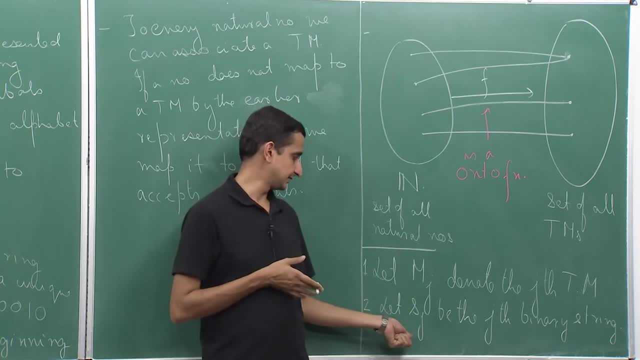 So I can just enumerate them. Okay, So let us say that s1 would be the string 0, or may be the string at the beginning of it. Okay, So s1 will be the string 0, s2 will be the string 1.. 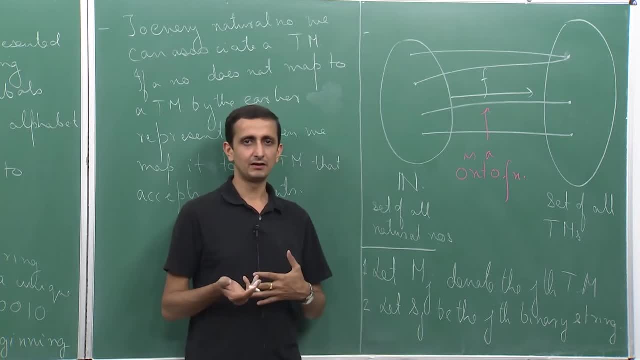 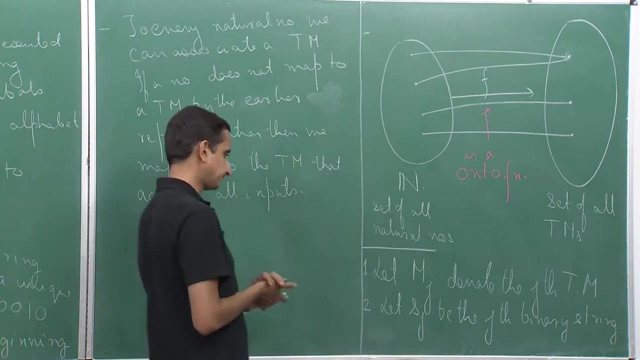 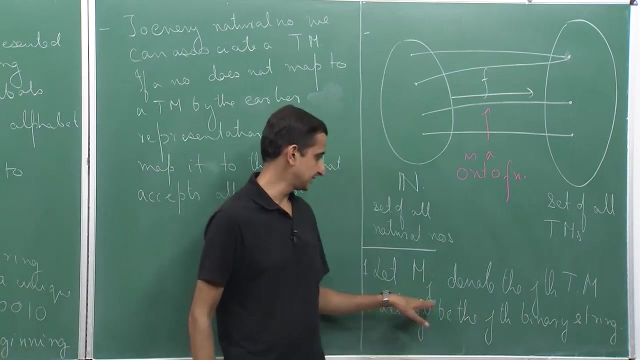 Okay, Then s3 will be the string 01, and then 10, and then 11, and so on. Okay, So I can basically enumerate all strings. So now that we have these two things, so we have an enumeration of Turing machines and. 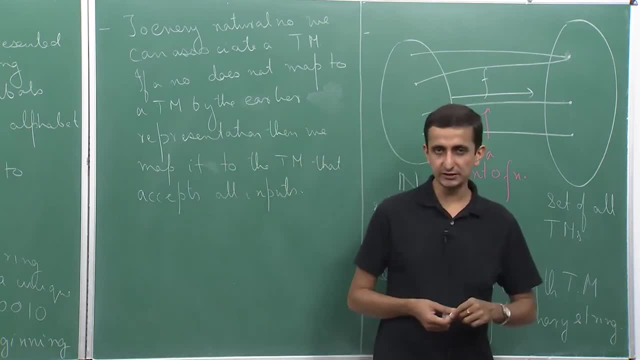 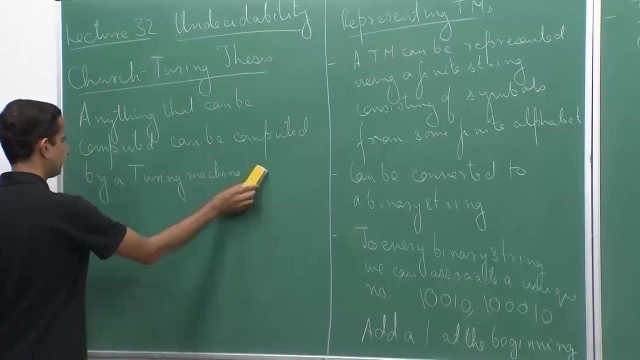 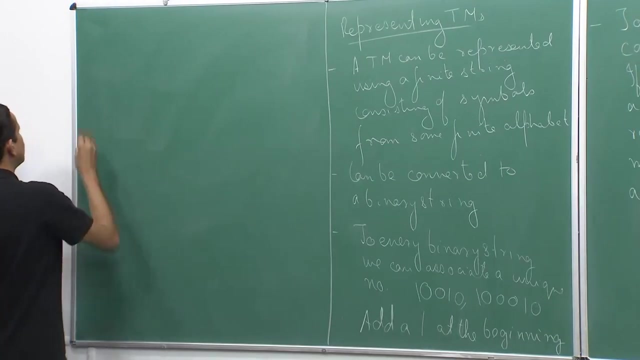 we have an enumeration of binary strings. Okay, So now we are in a position to talk about our first undecidable language. In fact, we will prove something more here. We will give a language that is actually not Turing recognizable, So a non-Turing machine. 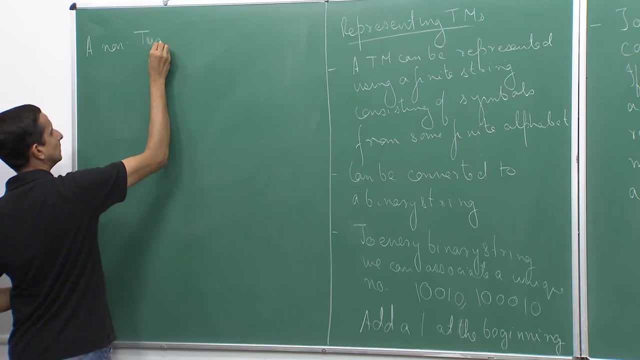 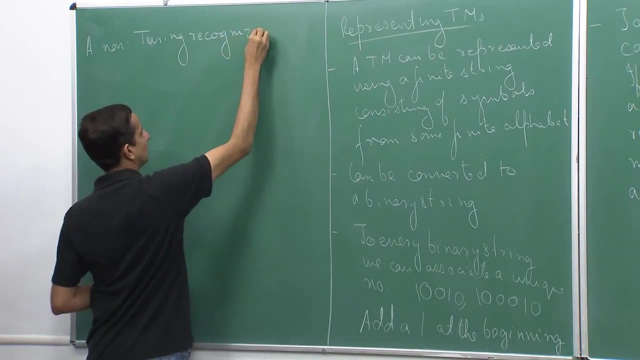 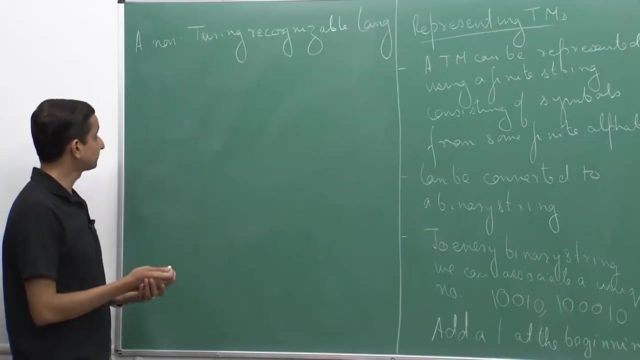 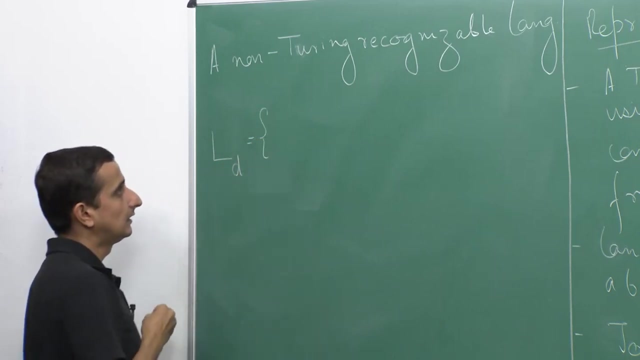 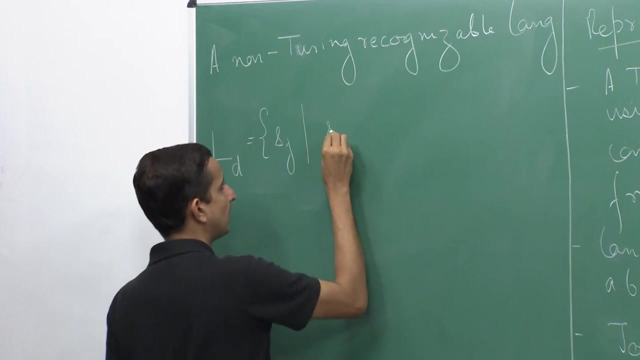 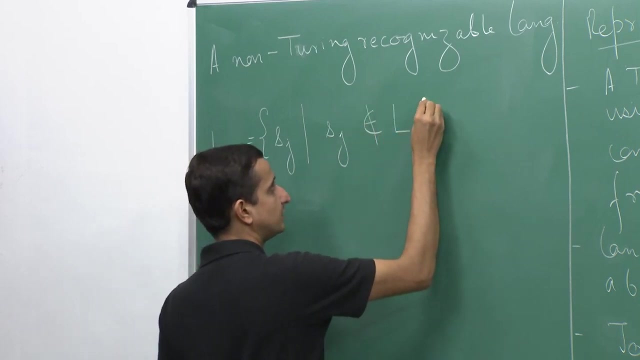 Okay, So now we are in a position to talk about our first undecidable language. Okay, So let us define this. So I define the language L D as the set of all binary strings s j. Okay, Such that s j does not belong to the language of m? j. 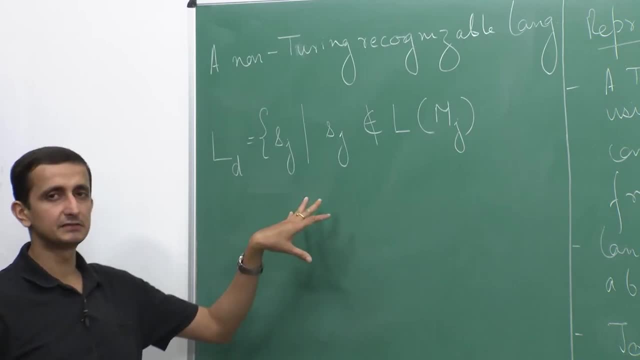 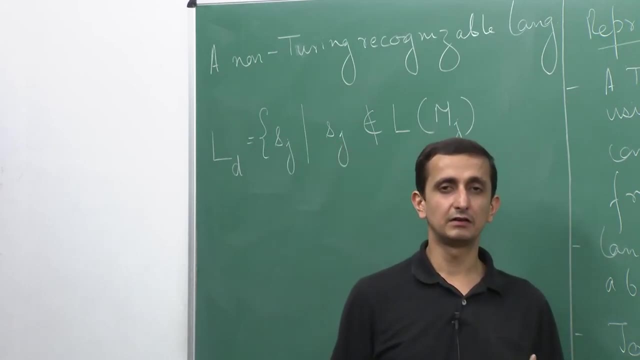 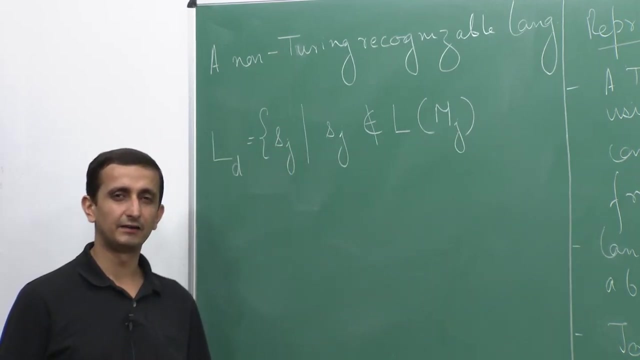 So this argument is what is famously known as the diagonalization argument. Okay, Okay, So this has been so. this was first introduced by George Cantor and later on it has been used by several mathematicians to prove various results. And this is the. I mean, this is the approach that Alan Turing took in his famous paper. 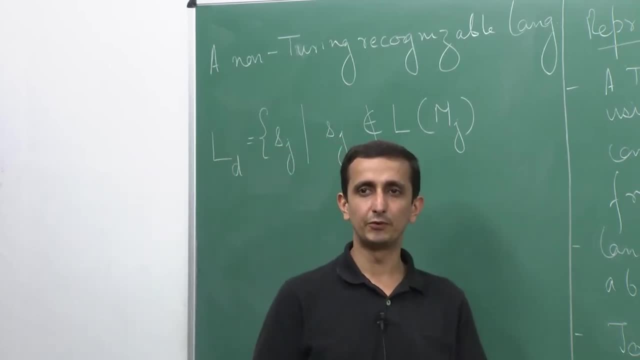 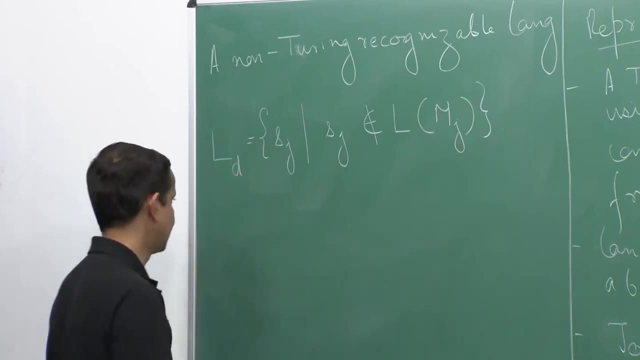 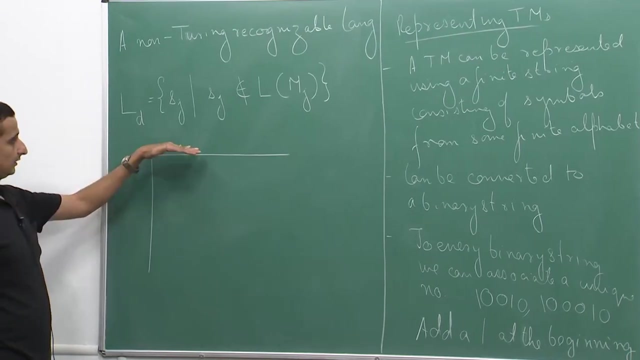 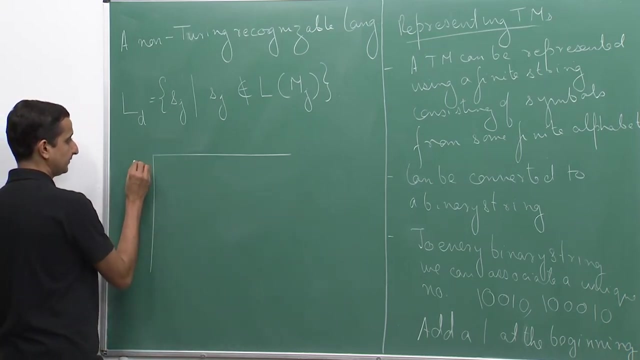 where he showed that there are problems that cannot be computed by a Turing machine diagonalization approach. Okay, So to understand this language, let me draw a table. Okay, So we have this semi-infinite matrix. So it is finite on the left and the top side, and on the right and the bottom it is infinite. 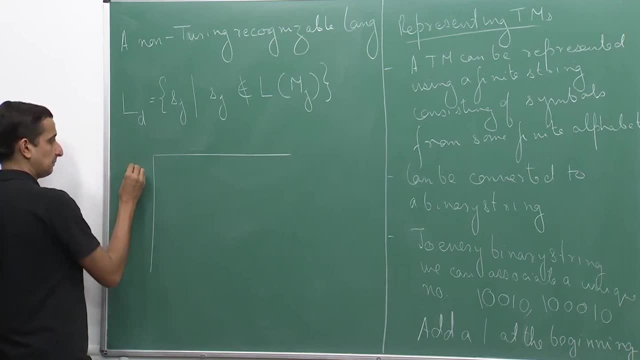 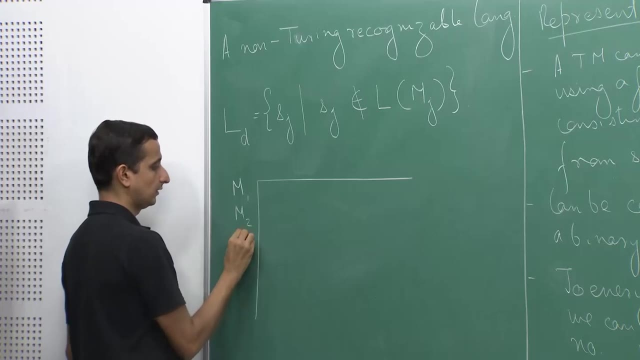 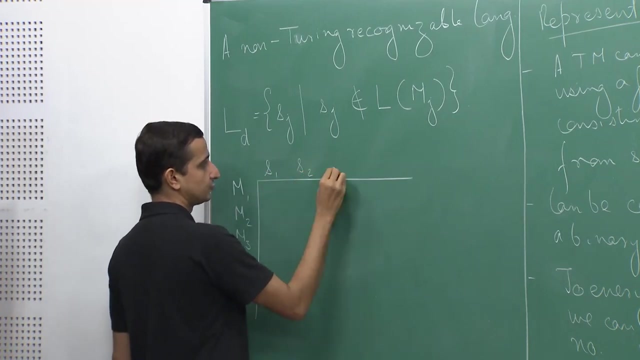 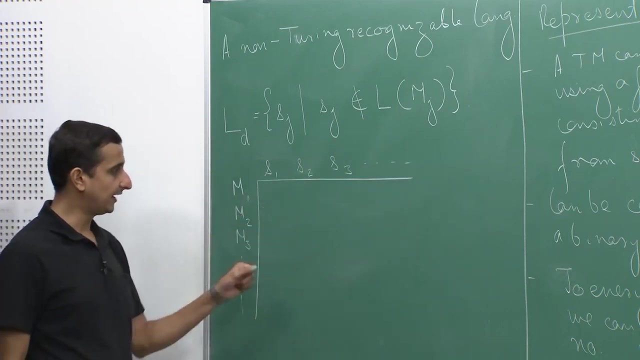 So on the rows I will put Turing machines. So first I will have m1, m2,, m3 and so on. Okay, And on the columns I will have the strings s1,, s2,, s3 and so on. And the way I fill it up, I fill up this matrix using 0 and 1.. 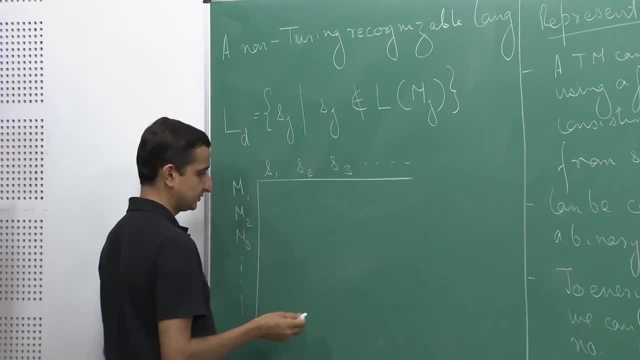 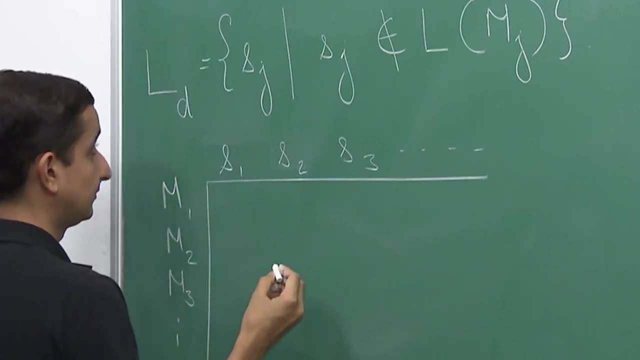 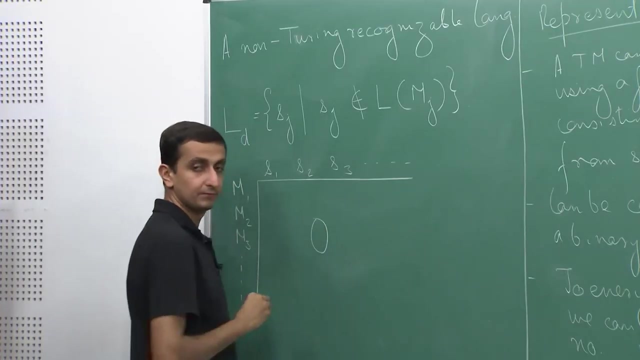 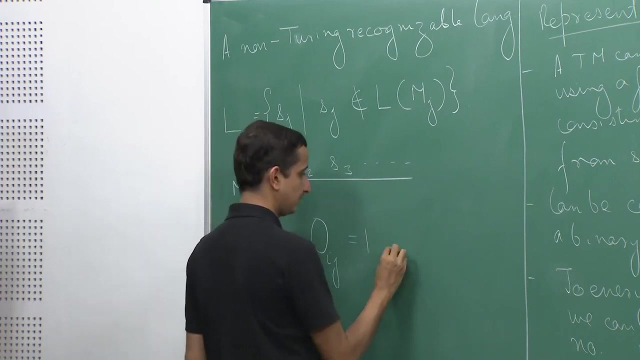 So I say that. so let us give this matrix a name, So I will call this matrix. let us say L, So let us give maybe not L, so I will call this matrix O. Okay, So O of i j is equal to 1 if m i accepts s j, otherwise it is equal to 0. 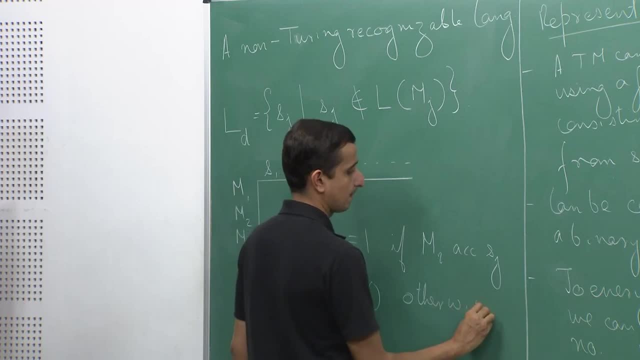 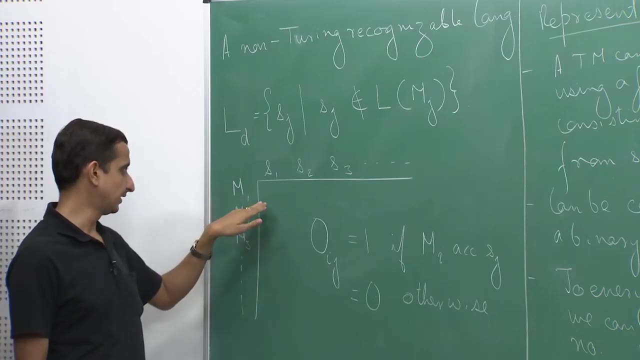 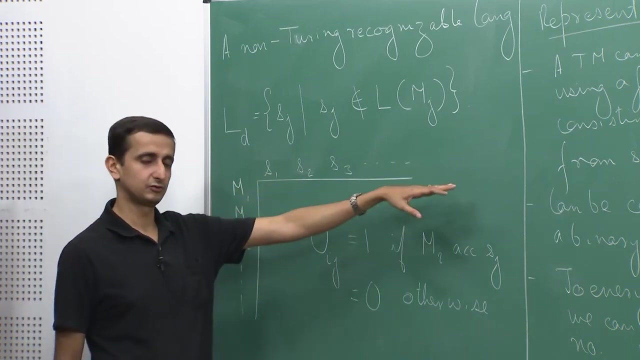 Okay, Okay, Okay. So essentially I look at this matrix. So I look at the first matrix, the first Turing machine, m1, I check whether m1 accepts s1, if yes I put a 1,, otherwise I put a 0, then I go to s2, s3 and so on. 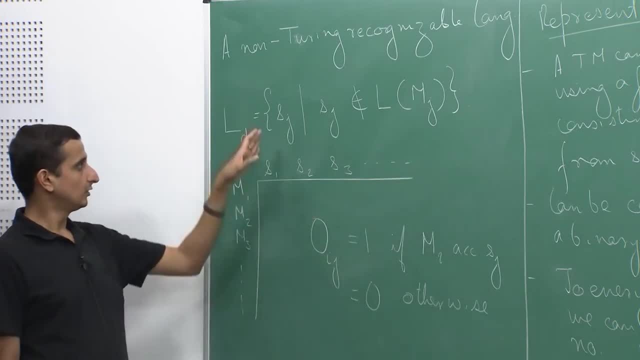 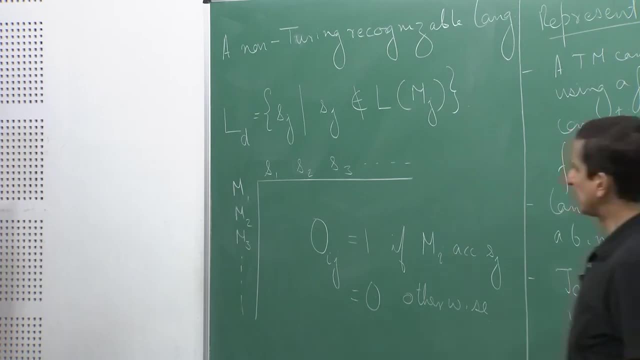 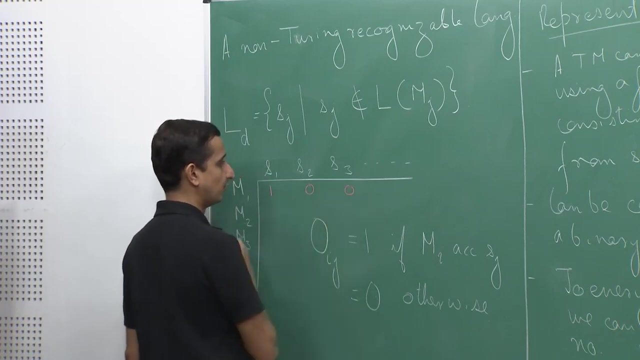 So I fill this up, then I fill the second row and so on. So the way this language LD is constructed is basically so, suppose, if I have a 1 over here. So let us say I have the following entries: 1, 0, 0, and then I have maybe 0, 1, 0, and then 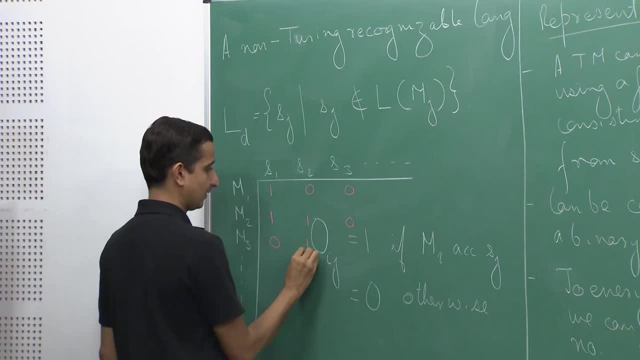 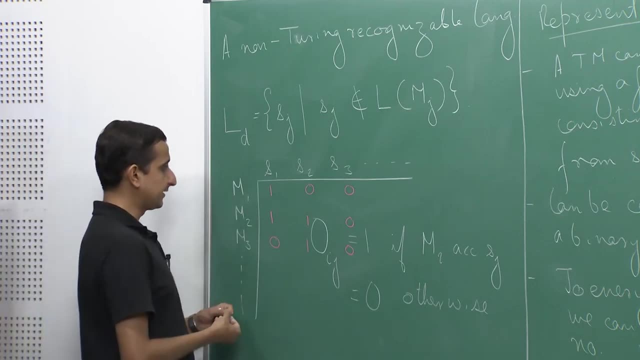 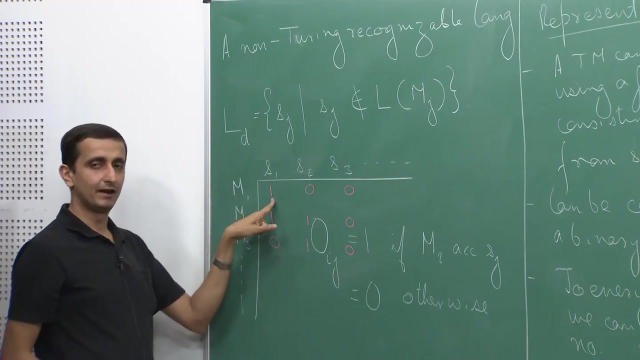 0, 1, 0 in this matrix. What I will do is that I will replace, so I will basically swap the entries of the diagonal. Okay, So I look at the diagonal of this matrix: If there is a 1, I flip it with 0, and if there is a 0, I flip it with 1.. 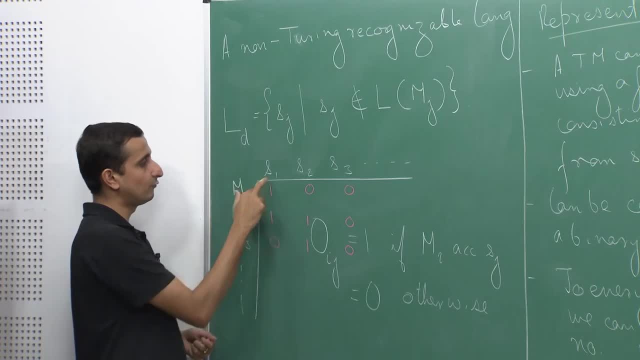 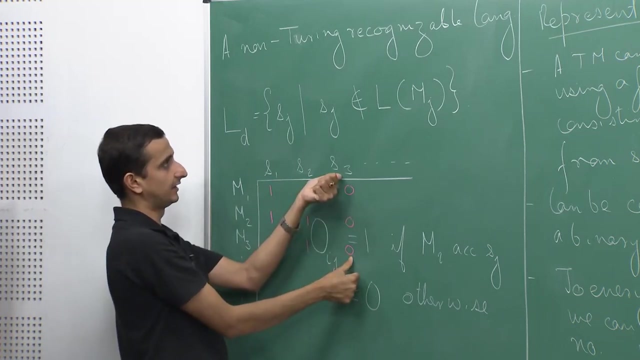 Okay. So in other words, if I have a 1 in the diagonal, it means that m1 accepts s1, in which case I will not add s1. So I will only add those elements of the diagonal which have a 0. So in this case, what we have is that m3 does not accept s3.. 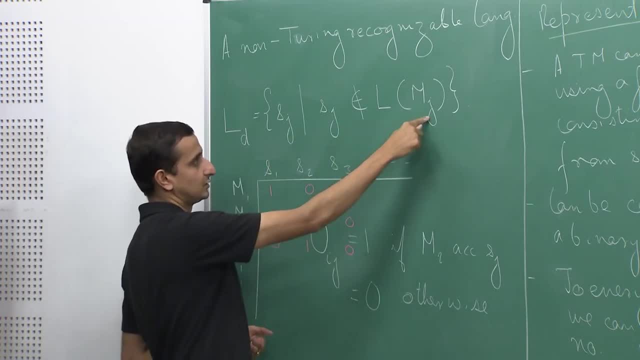 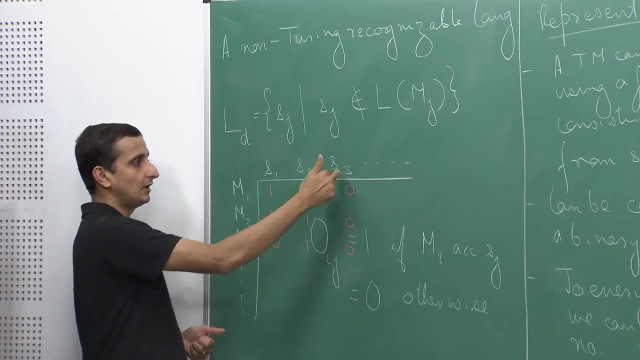 So basically, s3 is not does not accept s3.. Okay, So s3 does not belong to the language of m3, in which case we add s3.. So this is what we do, So we go through the diagonal. whenever we have a 0, I look at the corresponding string. 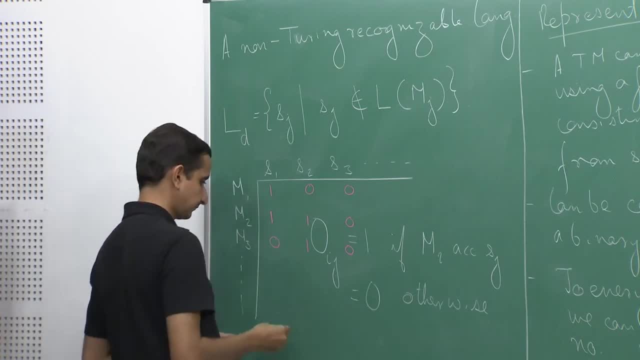 and I add it on to the language LD. Okay, So add strings sj, s1,, s2,, s3, s3, s4,, s5, s6, s7, s7,, s8,, s9, s9,, s10,, s11,, s12,, s12,, s13,, s13, s14,. 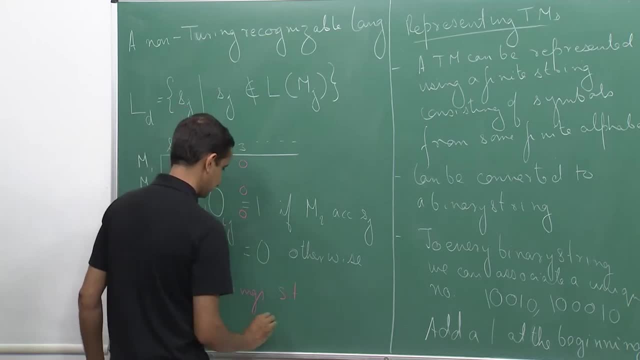 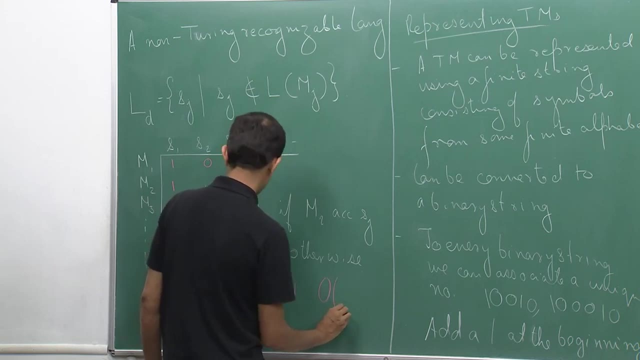 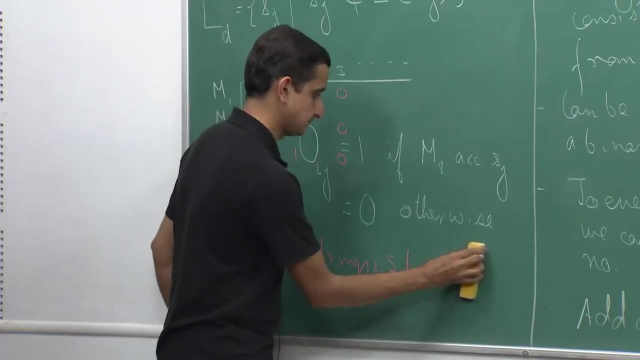 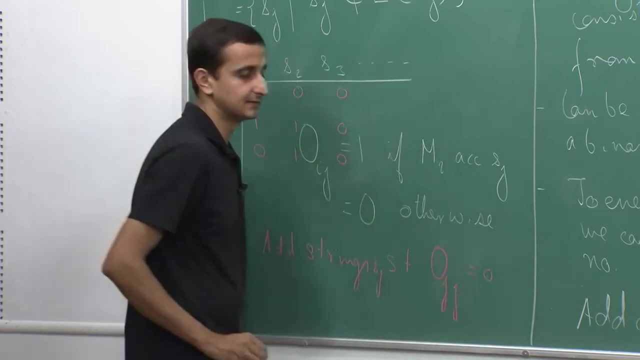 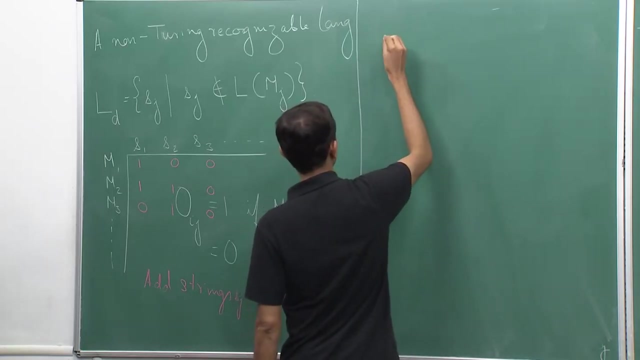 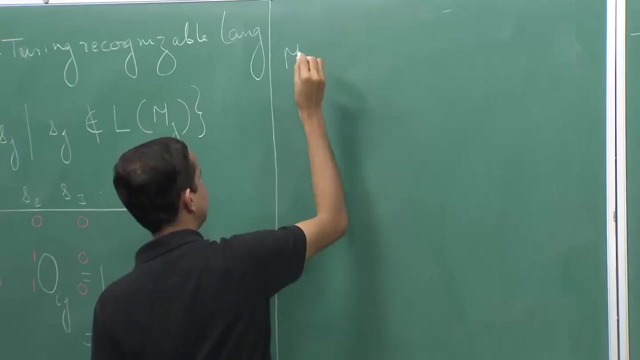 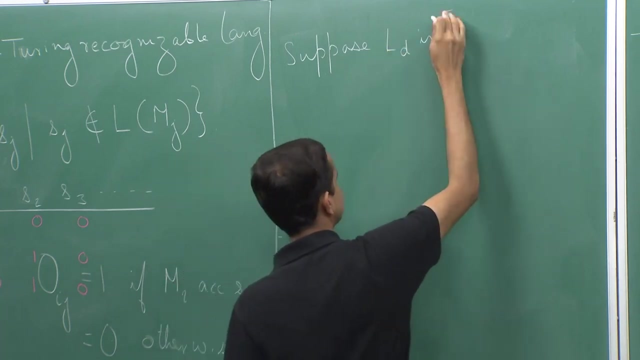 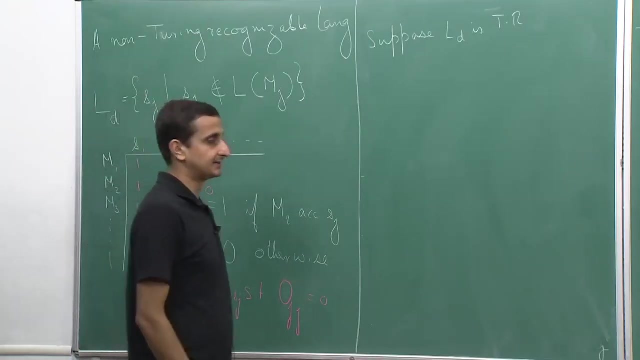 s14, sj, such that o jj is a 0.. Okay, Okay, Bye, Bye. So now that we have this, we can argue the following: So suppose, if Mj so suppose, Ld is Turing recognizable. So, for the sake of contradiction, let us say that Ld is Turing recognizable. 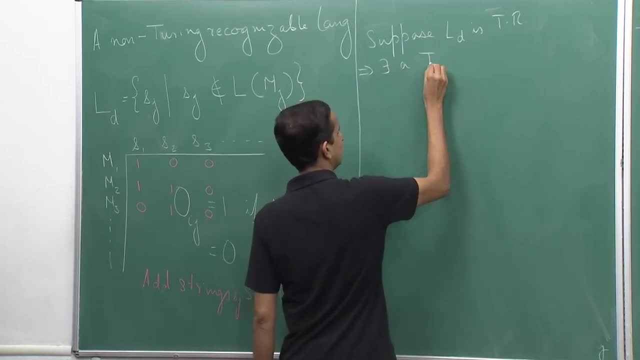 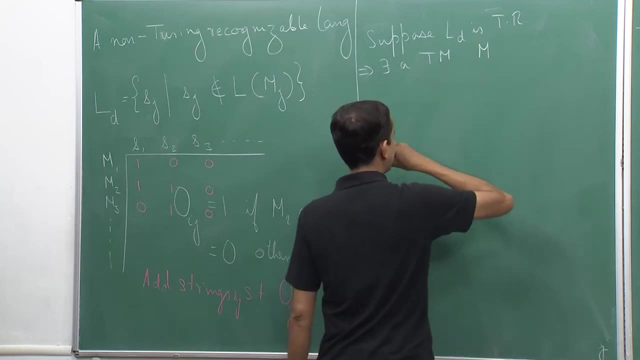 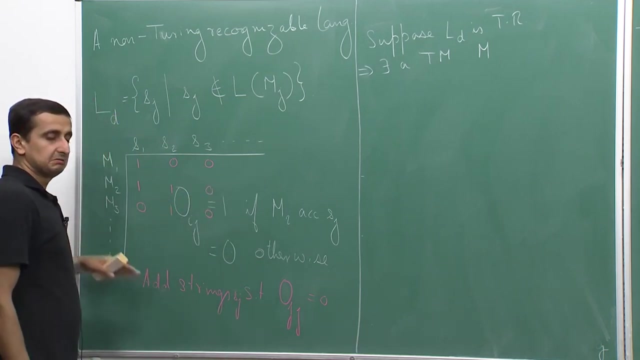 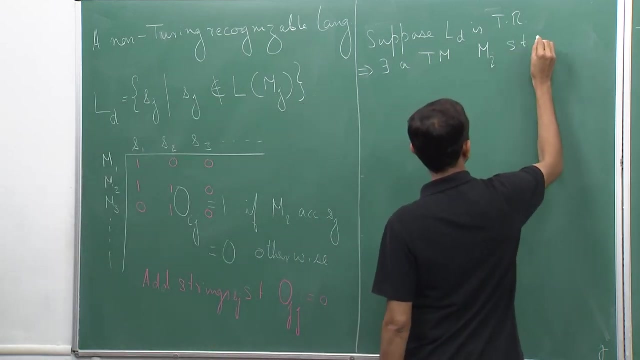 So then, there exists a Turing machine, let us call it M, and because I have enumerated all the Turing machine, this Turing machine must be the ith Turing machine for some i. So there exists a Turing machine, Mi, such that Ld is Turing recognizable. 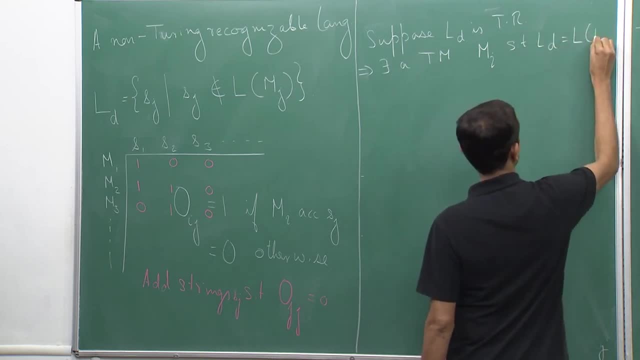 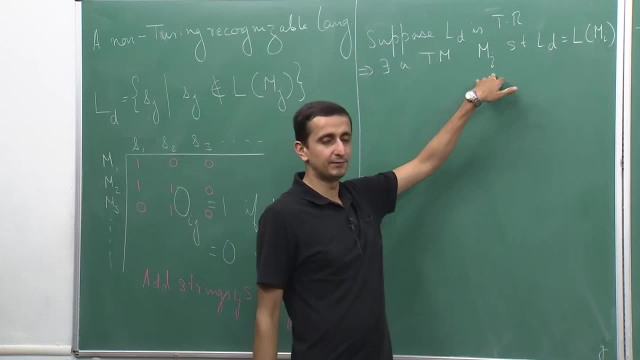 Such that Ld is equal to the language of Mi. So if this is Turing recognizable, it must be accepted by some Turing machine. That Turing machine is somewhere in the row. Let us say it is our ith row. So I say that Mi is the Turing machine. 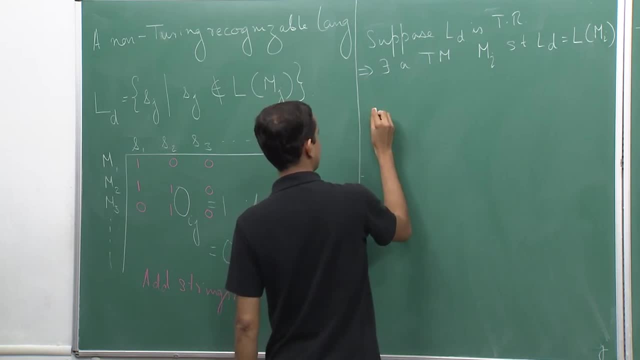 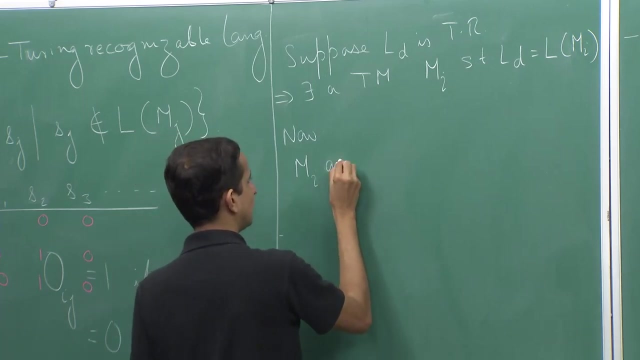 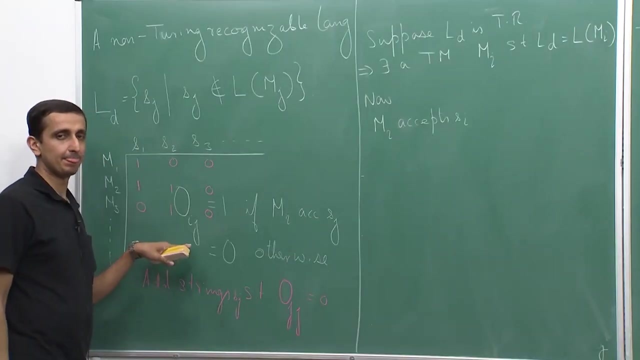 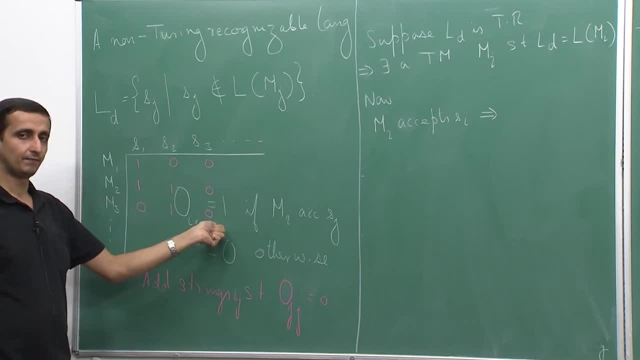 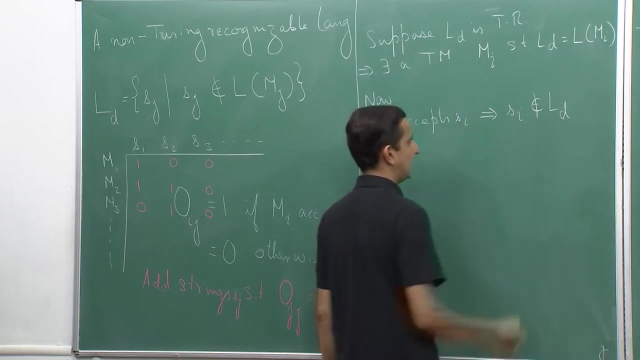 It means I have a 1, ok one on the table at that point, which means that by the definition of the Turing machine it should not belong to the language. So this implies that S i does not belong to the language L d because it only accepts those where the corresponding machine does not accept the 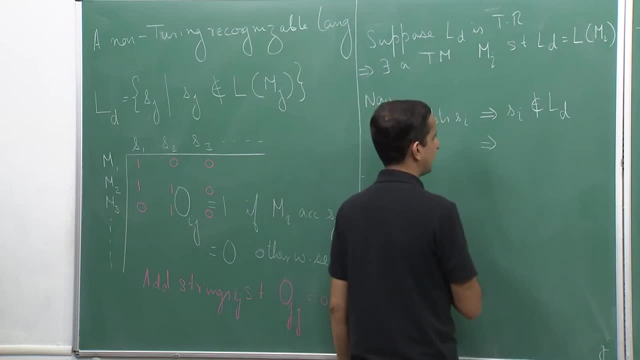 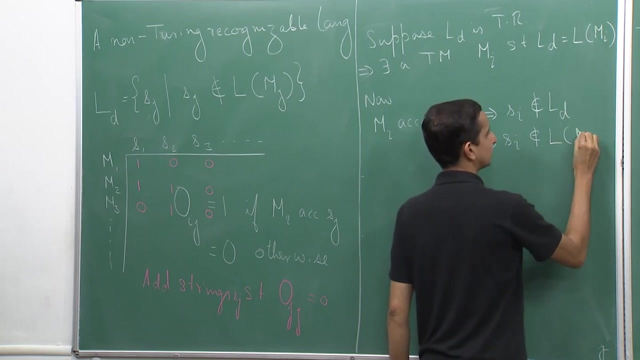 string. This implies that. so now, what is the machine? M i? M i is a machine for the language L d. So if S i does not belong to L d, then S i also does not belong to the language of M i, which implies that M i does not accept. 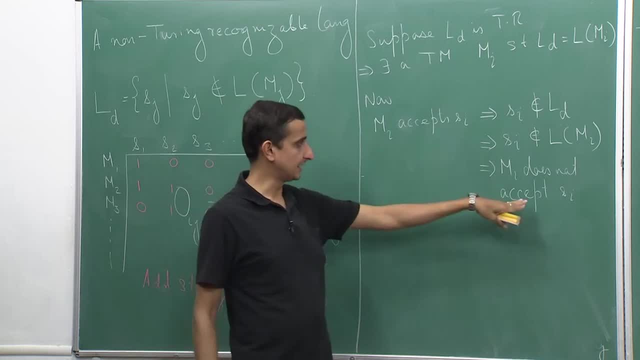 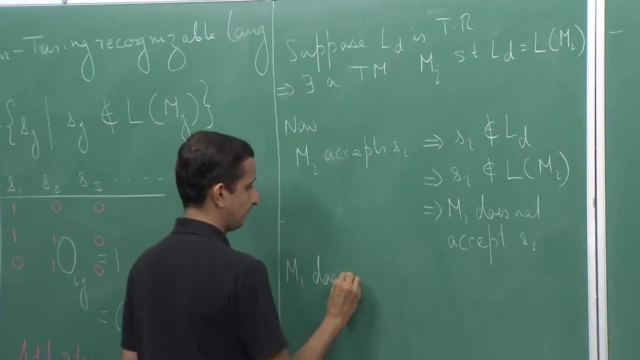 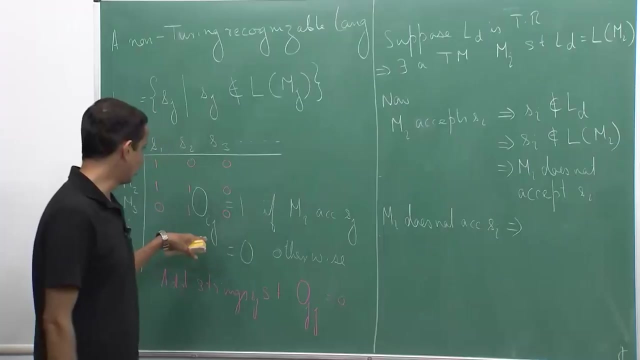 S i. So we have that if M i accepts S i, it implies that M i does not accept S i. Similarly, if M i does not accept that, Similarly, if M i does not accept that, If Mi does not accept Si. again, if I go to the table, I have a 0 over there, so I flip. 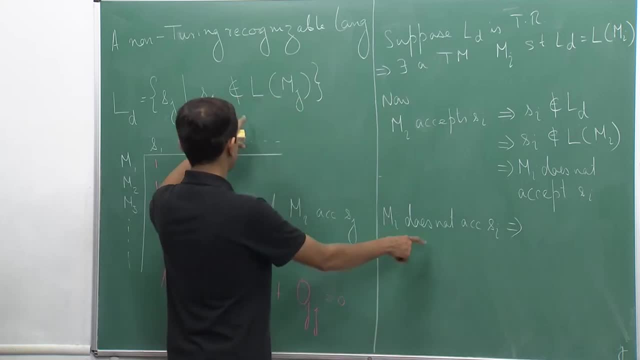 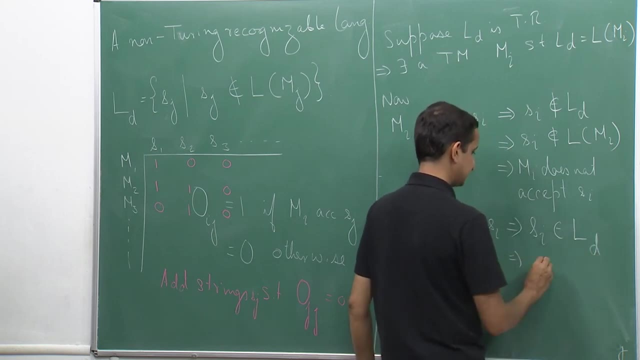 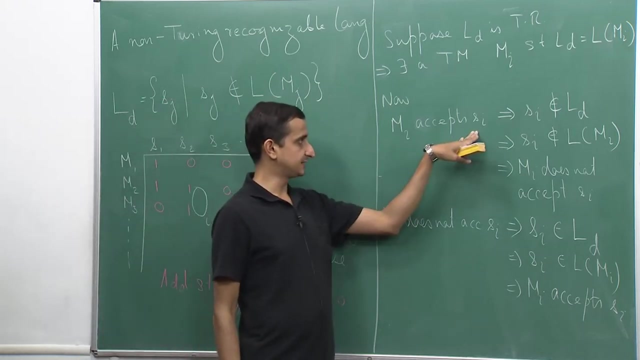 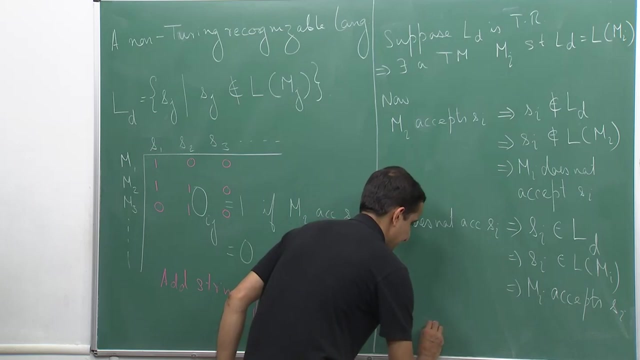 it to get a 1.. So if Mi does not accept Si, by the definition Si belongs to the language Ld, which means that Si is accepted by the machine Mi. so therefore we have a contradiction that if Mi accepts Si, if and only if Mi does not accept Si. so this gives us a contradiction. 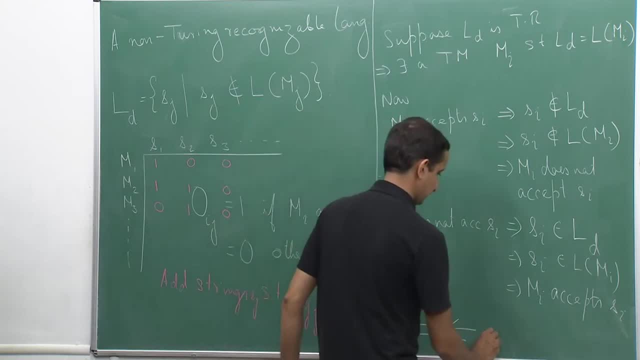 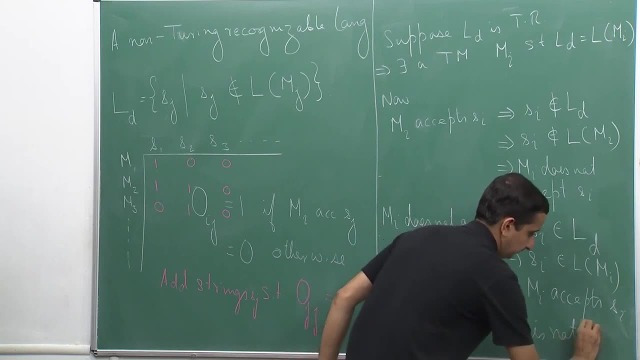 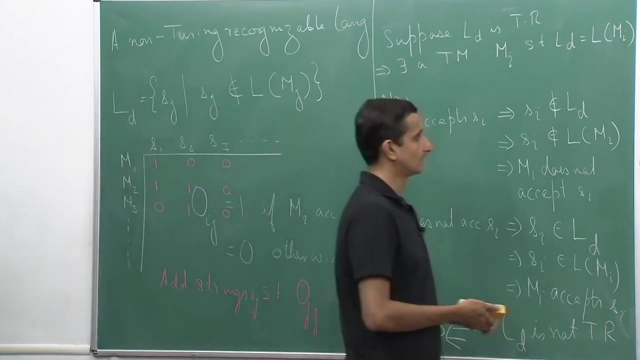 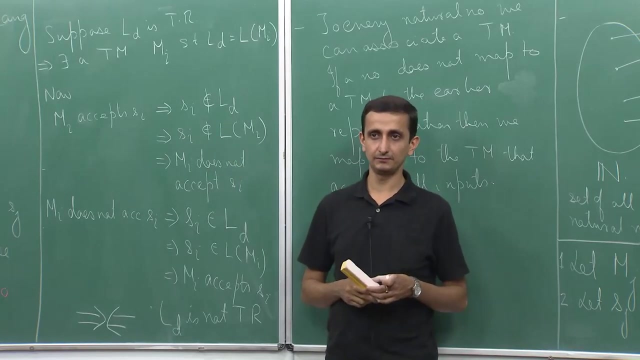 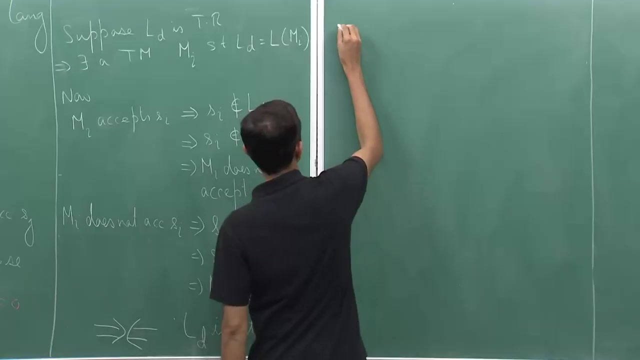 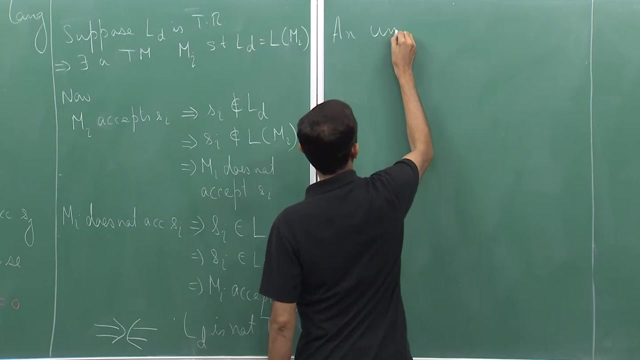 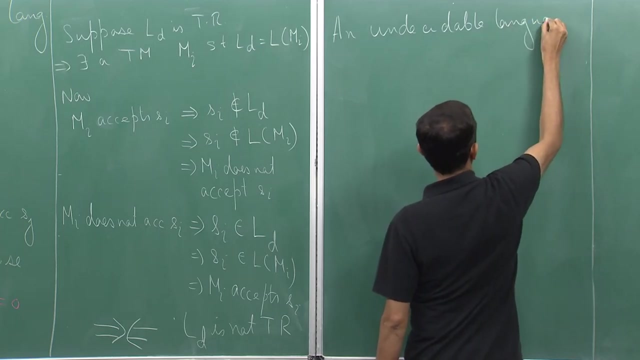 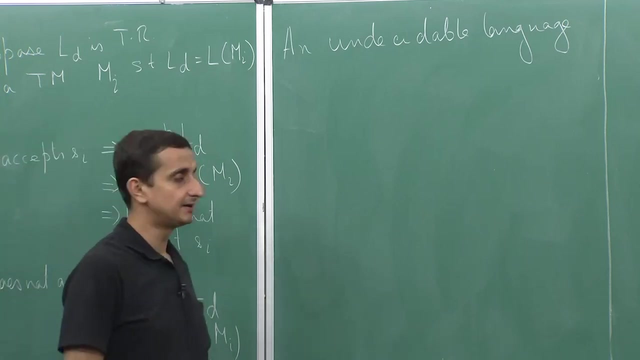 So therefore Ld is not Turing recognizable. So therefore we have exhibited a language which is not Turing recognizable. So next we are going to look at an undecidable problem. So in our next lecture we will prove that this language is undecidable. 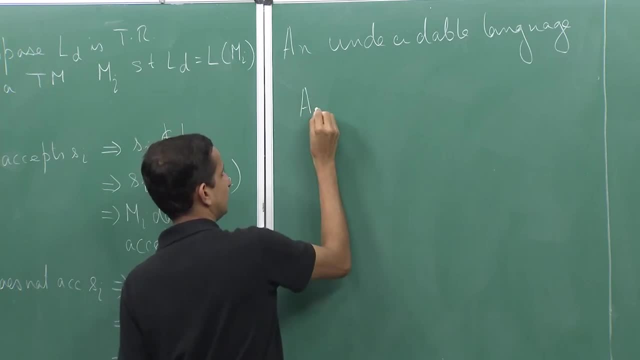 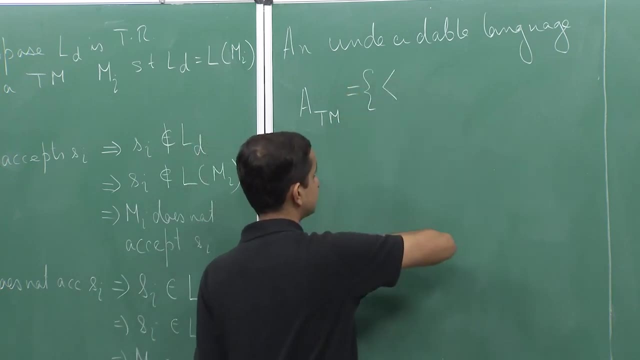 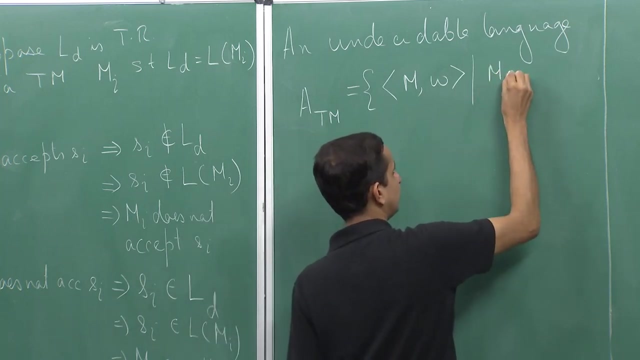 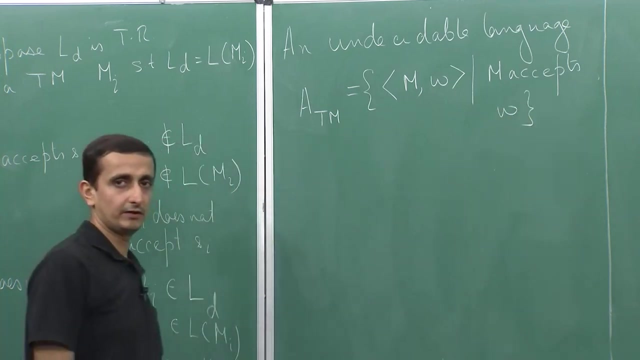 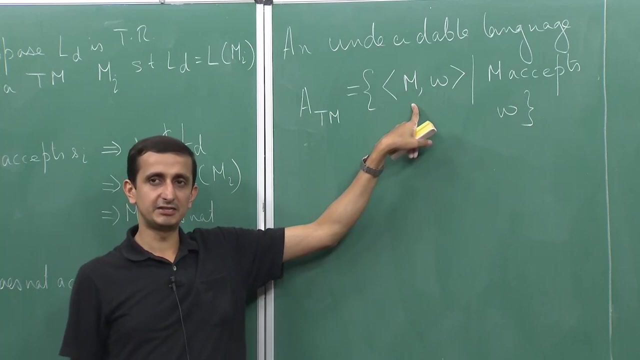 So the language that we are going to consider is. we define it as follows: So it is called Turing, It is an ATM and it consists of encodings of a machine, M and a string W, such that M accepts W. So this is a language which has an encoding of a Turing machine, M and a string. 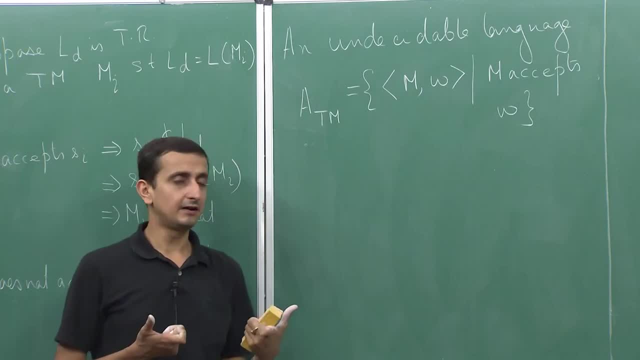 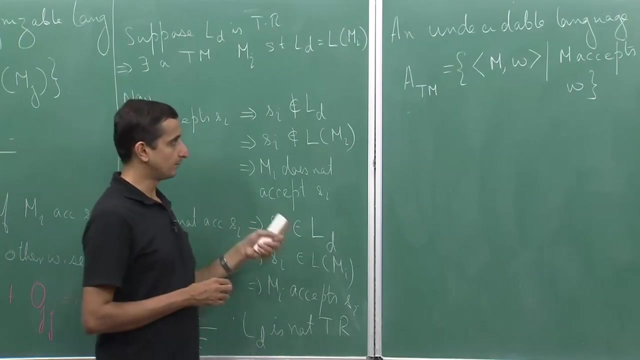 W. So they are given to it together And it consists of all those pairs such that the machine M accepts W. If M does not accept W, it is not in the language ATM. So in our next lecture we will prove that this is undecidable. 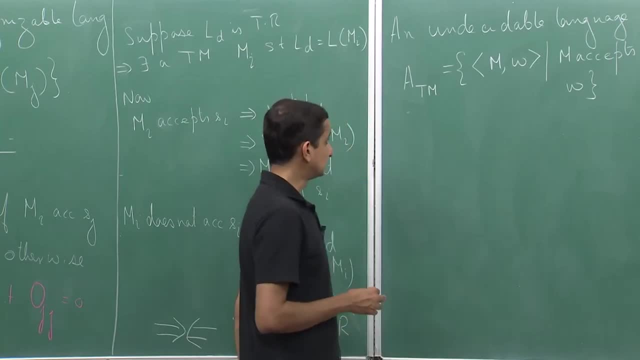 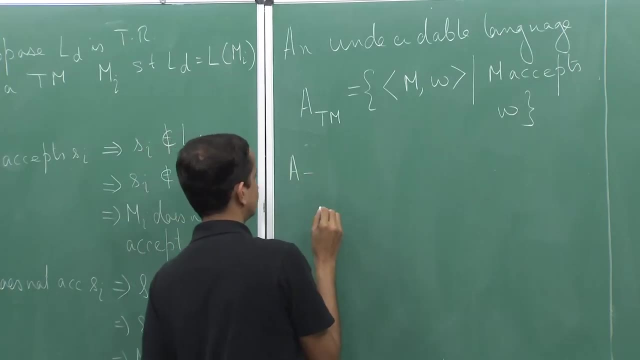 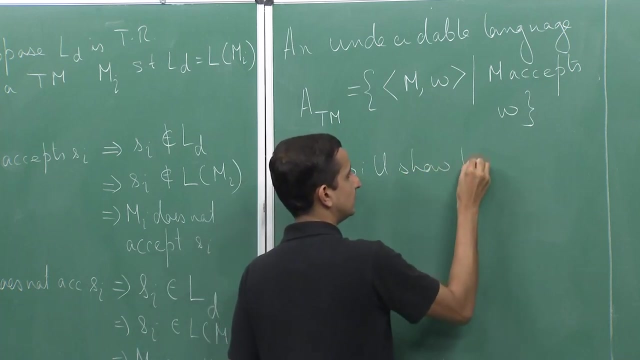 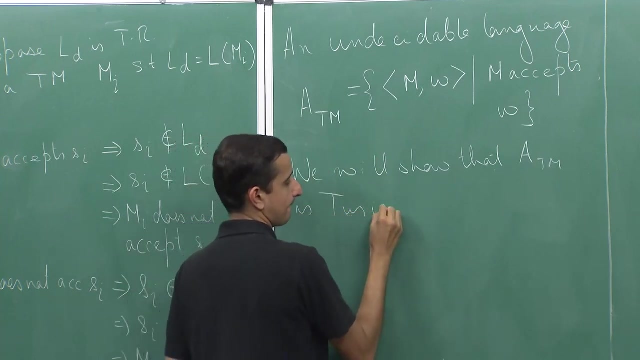 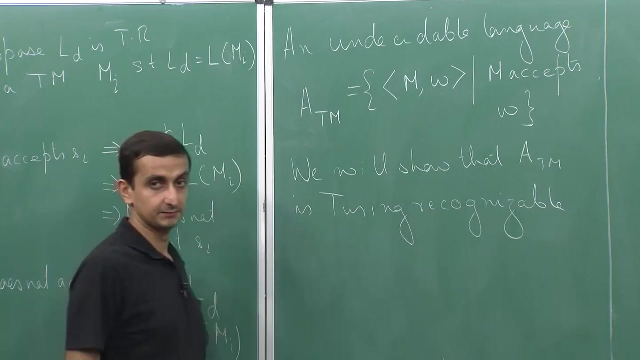 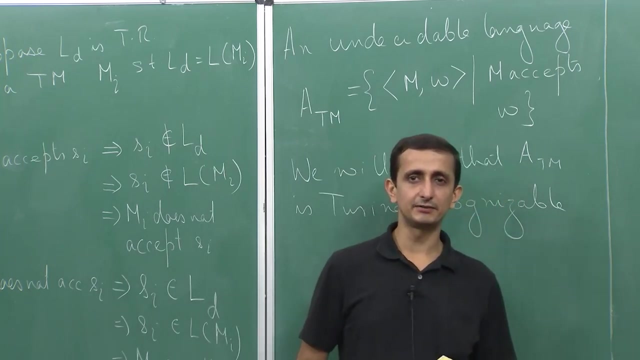 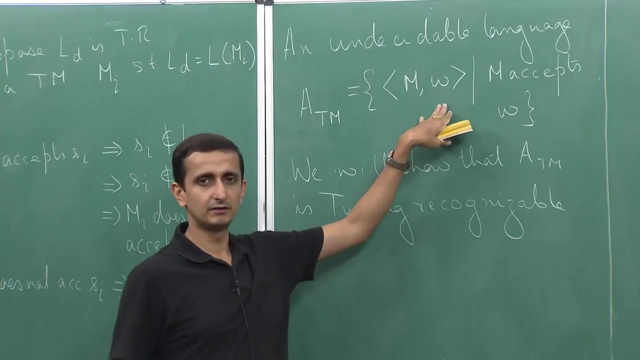 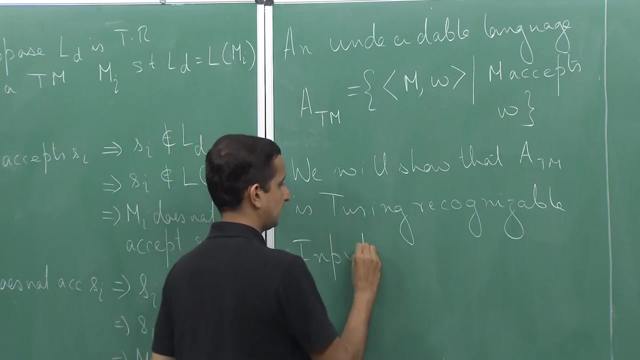 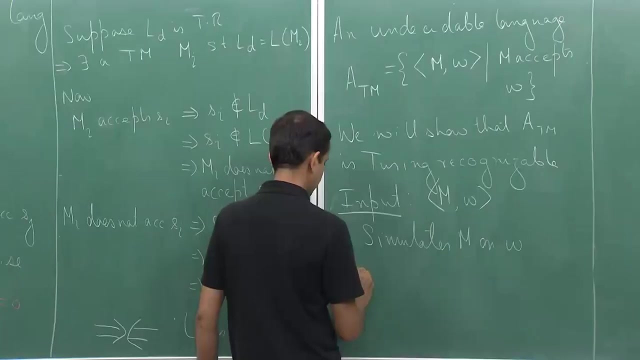 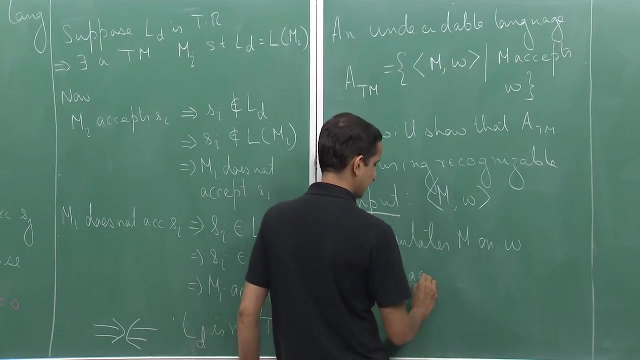 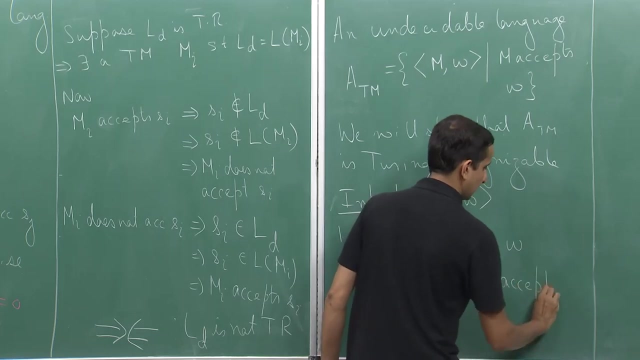 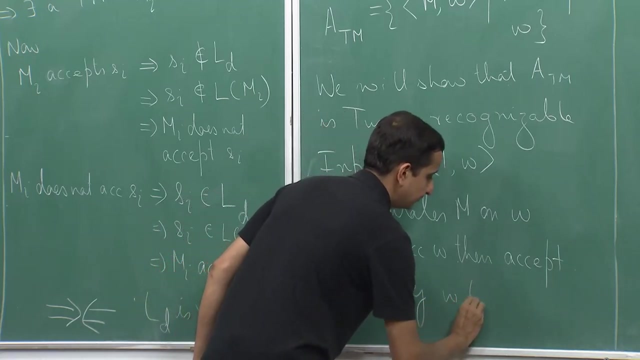 But what we are going to show today is that this language ATM is actually Turing recognizable. So If we accept W as a function of an PF, It can have a говорю M on W, And if M rejects W, then it tries to reset M. It is already over, because if her name is Monroe M or Monroe M, it cannot happen. 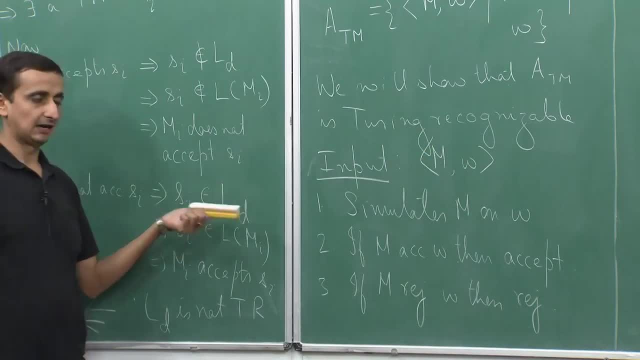 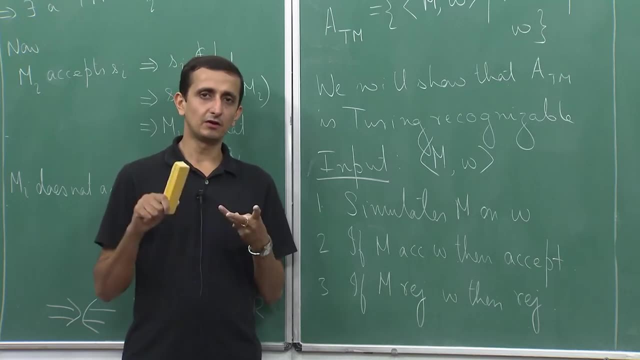 then just reject. So it is a very simple algorithm. So observe that when I simulate m on w, there are three possibilities: Either m can accept w, or it can reject w, or it can loop forever on w. So if m accepts w, then it accepts m. 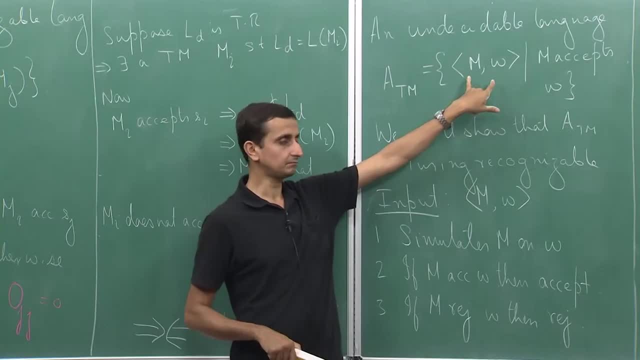 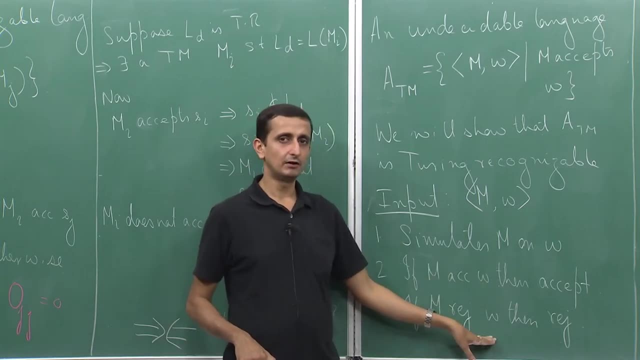 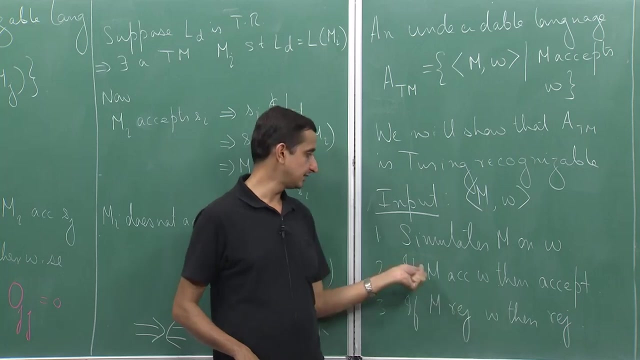 comma w, So it is according to. it is an instance which is in the language ATM. If m does not accept w, if m rejects w, then anyway I am rejecting, So it is not here. And if m loops forever on w, then anyway the first step never stops, So the first step goes on forever. 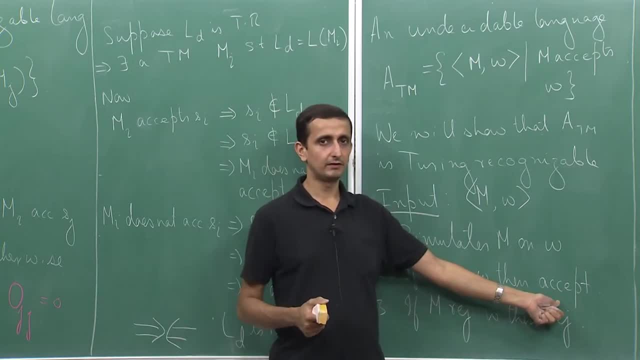 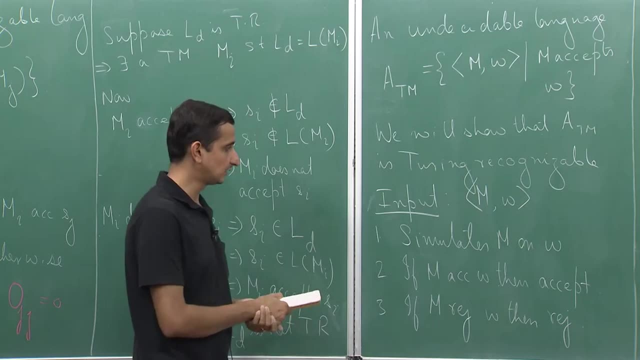 in which case also, I do not accept. Hence it is not in the language ATM as required. So what we will show in the next lecture is that ATM is not only, it is, certainly it is- Turing recognizable. So it is not in the language ATM. So it is not in the language ATM. So it is not in the